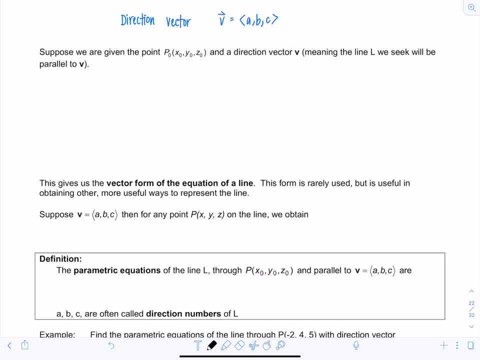 think about what sort of information we have and what's true about the line. okay, So we're in three-space, okay, So here's my x-axis, z-axis, y-axis. okay, And I'm given some point p-naught, I'll put it here, okay, And then I have a direction vector. 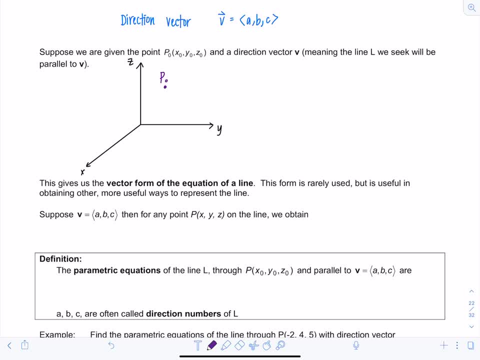 v, and I know that my line is parallel to this direction vector. So let's say vector v. it's going to be a position vector, maybe it's something like this: Here's my vector v. okay, Now the equation of the line would contain all points, so all x, y, z, right? 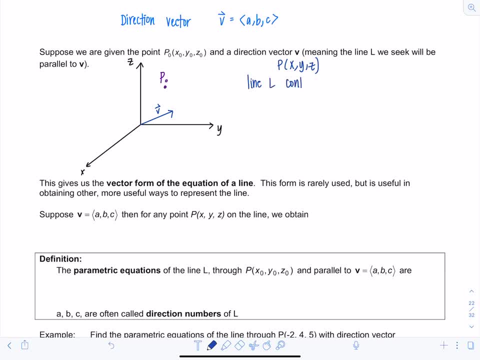 would be on my line l, So it contains all the points p, x, y, z, such that p-naught, y-naught and z-naught. So the vector from p-naught to any other point p is parallel to v. So let's draw that out and see what that would look like. 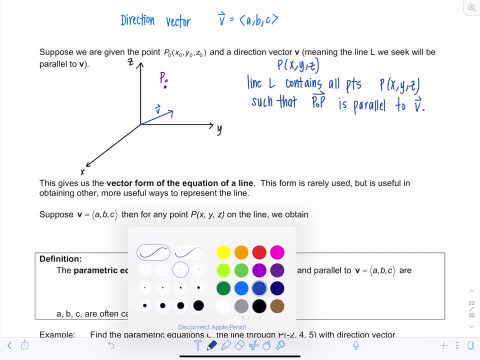 So think about if you were to have some line l right parallel to this vector v. it would look something like this: right, This is my line l And any other point p here on this line line. this vector from p-naught to p needs to be parallel to v. Well, what do we know about? 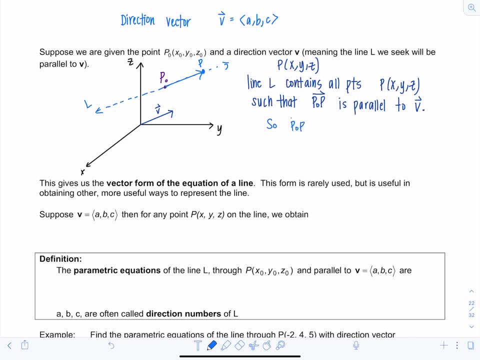 parallel vectors. So that means p-naught p is going to be a scalar multiple of v. So I can write the vector p-naught p as some scalar. We'll use t times v, So t is a scalar. So now I can call this vector here. let me darken it a little bit. 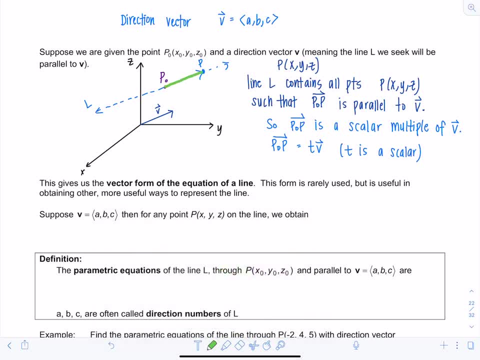 So this vector here, from p-naught to p, that vector there is going to be tv right. It's a scalar multiple of the vector v. They're not necessarily the same length but they're parallel. Okay, well, notice, here we have an. 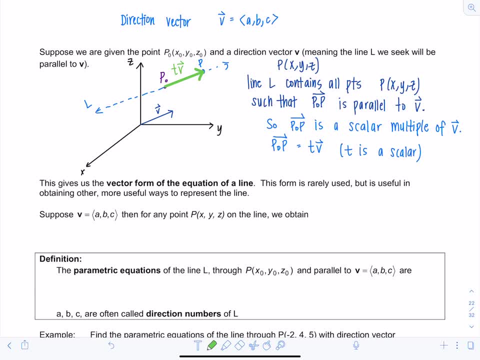 integral of v, So t is a scalar multiple of v, So t is a scalar multiple of v, So t is a scalar interesting relationship between position vector that goes to p-naught and position vector that goes to any other point on the line. So I'm going to call the position vector to p-naught r-naught. 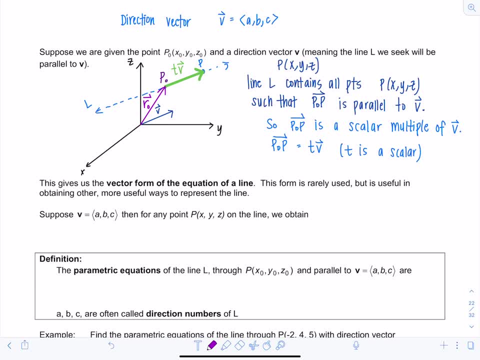 And then I can write a vector position, vector to any other point on the line. I'll take it to p here And I'm going to call that vector r. Now notice that r-naught plus t times v is equal to r. Can you see that? I'll draw in that addition. 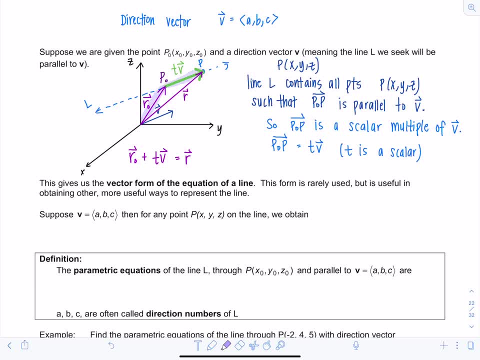 So I have r-naught, I add tv and the result is the vector r, And this holds for any vector r that connects a point on the line to the origin, So for any position vector that terminates on the origin. And this in particular gives us: 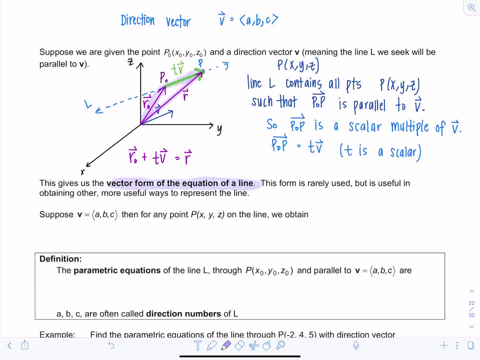 the vector form of the equation of a line, And this form it's rarely used, but conceptually it's how we build the idea of how to write the equation of a line in three space. okay, So there are more useful ways that we're going to rely on primarily for the remainder of the 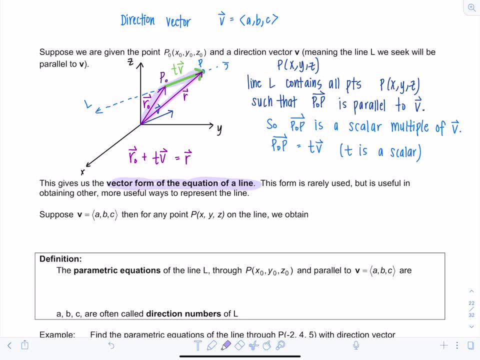 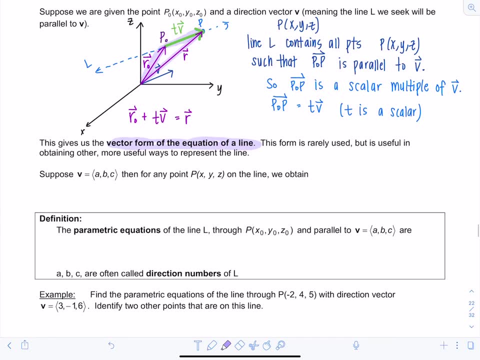 course, but this is the first one, since we understand where it's coming from. So suppose we have direction vector v with components a, b, c, Then for any point p, x, y, z on the line, we obtain the following: So my vector r. I'm going to write it the other way around now. So 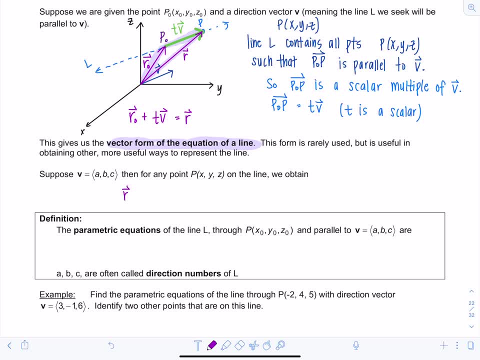 I'm going to have remember we have: r is equal to r naught plus t, v. But this basically becomes remember: r was the position vector to any point on the line, so I could write it as x, y, z. 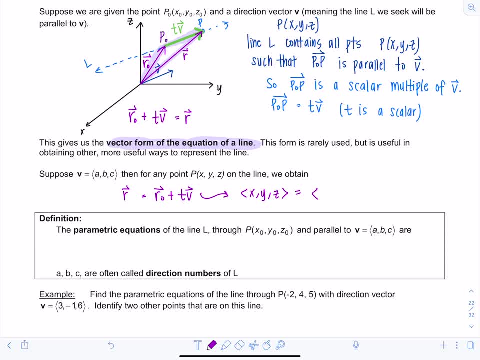 in component form equals r naught. I could write as: x naught, y naught, z naught, plus t, v, T times. vector v had components a, b, c. okay, And then the parametric equations of the line L. 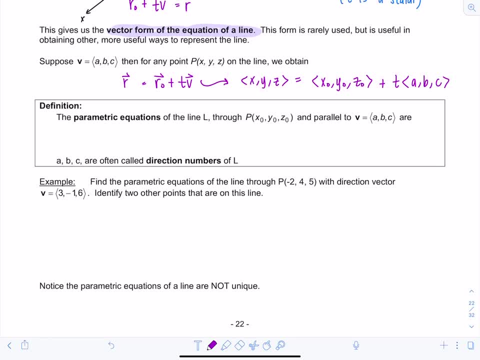 through the point p- naught, with coordinates x naught, y naught, z naught, and parallel to direction, vector v, a, b, c is given as follows: So you obtain the parametric equations by setting all of the corresponding components equal to each other. So we would have: x is equal to x naught. 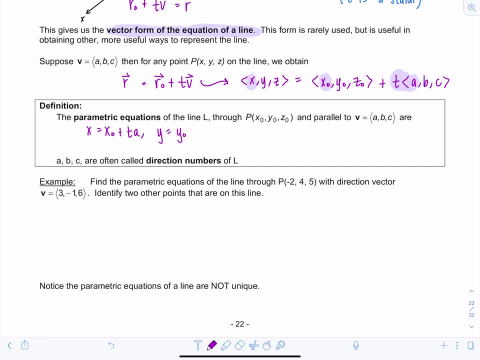 plus t a, y is equal to y naught plus t times b. And then z is equal to z naught plus t times c, And this is probably the most popular form of writing the equation of a line that we're going to work with. a, b and c are often called the direction numbers of the line L. okay, 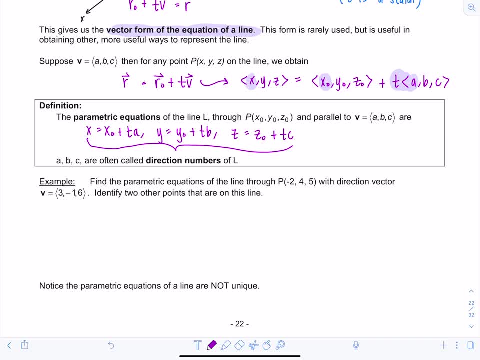 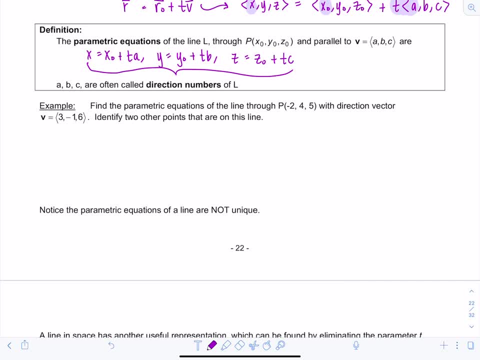 Okay, so here we go. So parametric equations: x is going to equal x, naught, which is negative, 2, plus 3 times t. Don't write t3,, that looks weird. y is equal to y, naught, that's 4,. 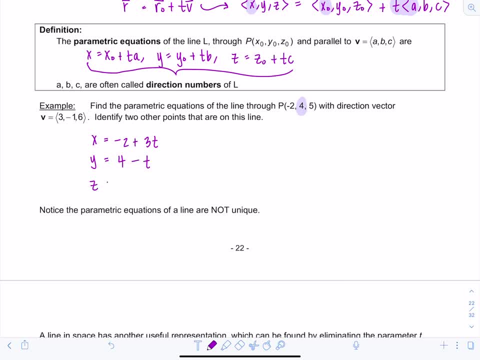 minus 1 times t, And then z is equal to z. naught that's 5, plus 6t. So here's our parametric equations. You can generate all of the points on the line by changing the values of your parameter. 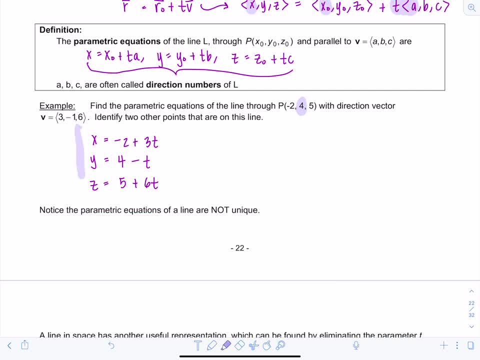 Okay, that box is just not working for me, is it? Okay, here we go. So t can be any real number, And so, as you let t vary, it'll generate all the points on the line. So the problem asks us for two. 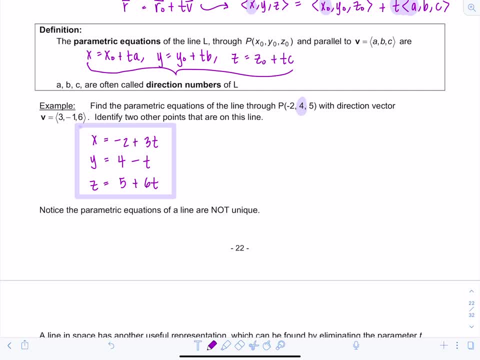 other points that are on the line. you could pick whatever you want to plug in for t to obtain them. Don't plug in t equals zero, because that's just going to give you the initial point that you use. So pick something other than zero. So say we're going to use t equals 1.. 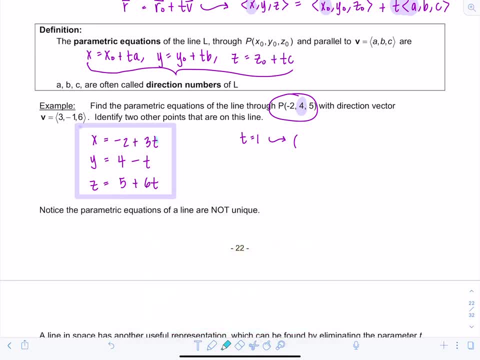 Then I'd obtain the point. So I'm substituting in 1 for t now to get the coordinates of another point on the line. So negative: 2 plus 3, that's 1.. 4 minus 1, that's 3.. 5 plus 6, that's 11.. 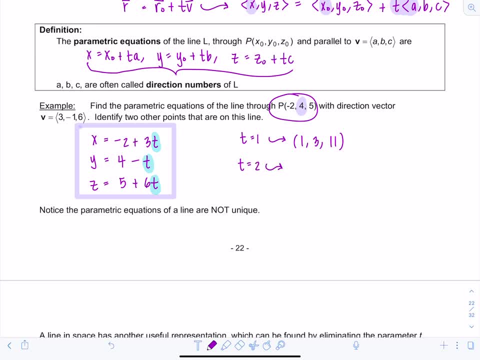 And then we need one more. So say we do t equals 2. Then we'll get negative 2 plus 6, so 4.. Next component would be 2.. And the last one would be 5 plus 12, so 17.. So those are two other points. 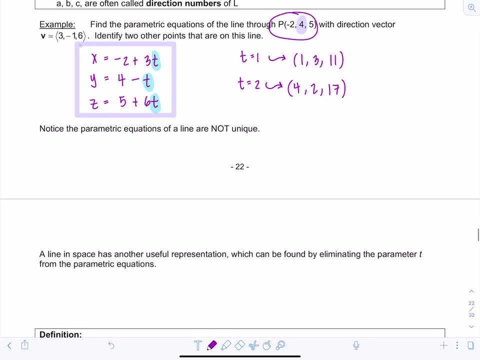 Okay, now notice that the parametric equations of a line are not unique. If, instead, we had chosen our initial point to be maybe 4,, 2,, 17, right, which we know lies on the line We just came up. 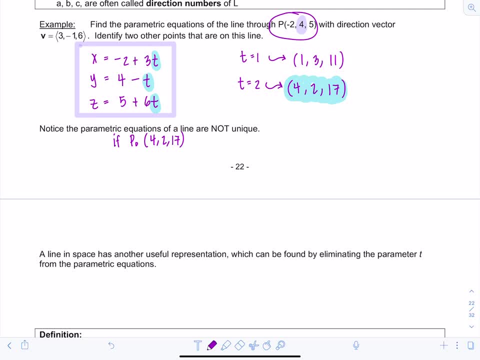 with that point right now, My parametric equations would look different. The direction vector is the same, But now I would have x equals 4 plus 3t, y equals 2 minus t and z equals 17 plus 6t. 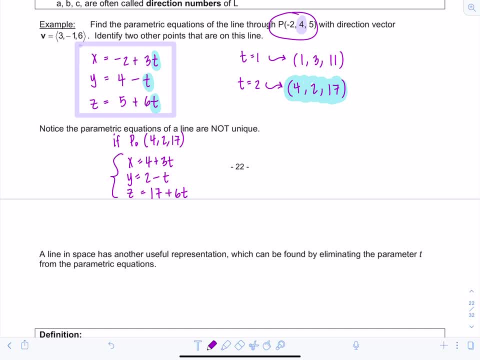 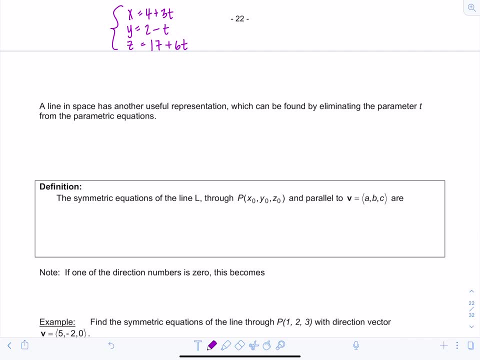 So notice it can be a little tricky because you can have more than one set of equations to represent a line. Now a line in space has another useful representation which can be found by eliminating the parameter t from the parametric equations. So we know that we have x. 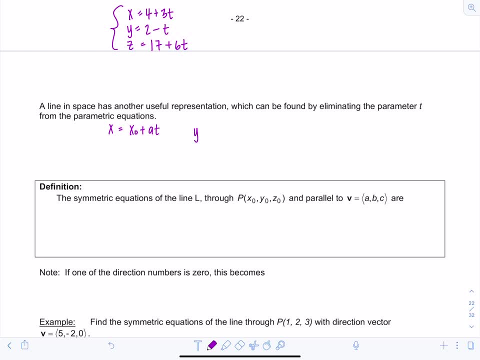 equals x, not plus at, and then y equals y, not plus bt, and z equals z, not plus ct. Well, if I solve for the parameter t, I would get: x minus x, not divided by a, is equal to t. 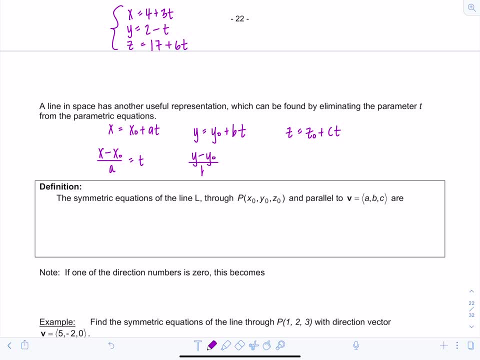 Similarly, y minus y, not divided by b, is equal to t. And then, lastly, z minus z, not divided by c, is equal to t. And so I know all of these quantities here, since they each are equal to t. 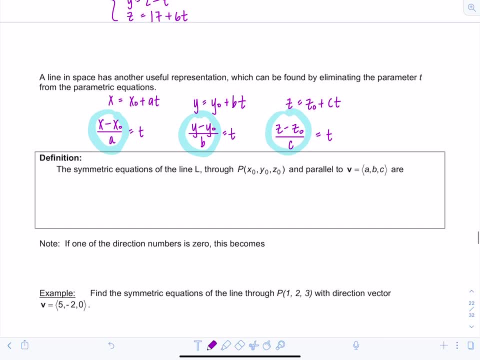 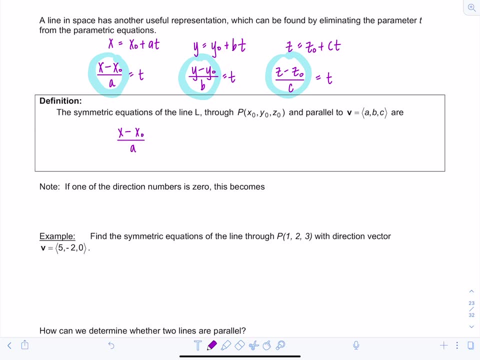 must be equal to each other, And that's where we come up with the symmetric equations of a line, And they're as follows: So you would set them all equal to each other. So x minus x naught over a is equal to y minus y naught over b, which is equal to z minus z naught over c. 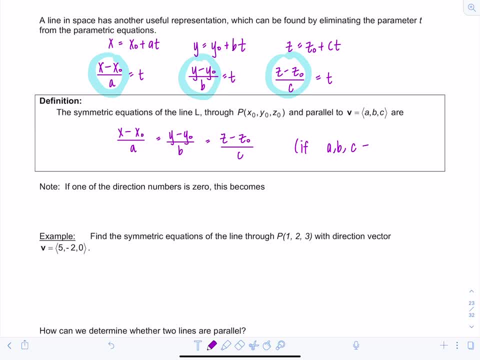 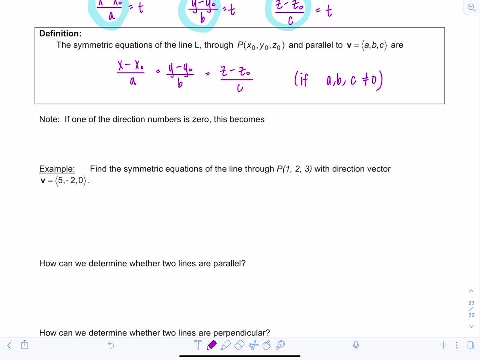 provided a, b and c are different from zero. Okay, Now what if one of the direction numbers is zero? right, That's totally possible. So what would you do in that case? Well, you would only use the symmetric equations for the direction numbers that are non-zero. So for 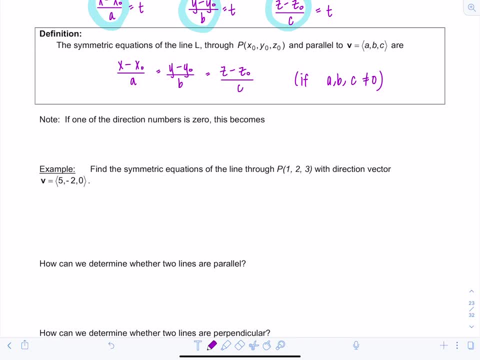 example- I'm just going to assume b is zero, just to give you a hypothetical- You would write: x minus x naught over a is equal to z minus z naught over c. And then you would say: ps y is equal to y naught, Because if the direction 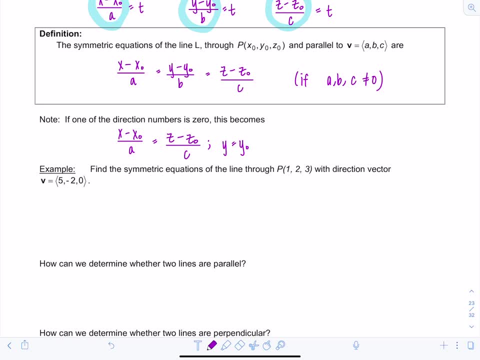 number for that component is zero, then that means it's just going to be equal to. every single point on the line is going to have the same coordinate as the initial point that's given, And this would be in the case if b is equal to zero. Okay, Good, So here we go Find the symmetric equations of: 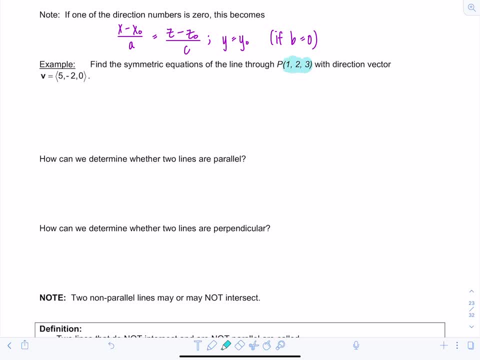 the line that goes through the point one, two, three, with direction number zero, Direction vector v: five negative, two, zero. So notice here: since I have a zero for the third component, that means separately- I'm going to write the equation: z is equal to three. That: 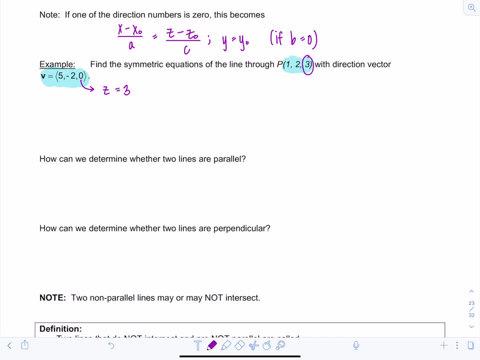 coordinate will not change for any of the points on the line, So the symmetric equations would just be: x minus one coming from here, divided by five, is equal to y minus two divided by negative two. Then you would write the equation: z is equal to y minus two divided by negative two, and then you: 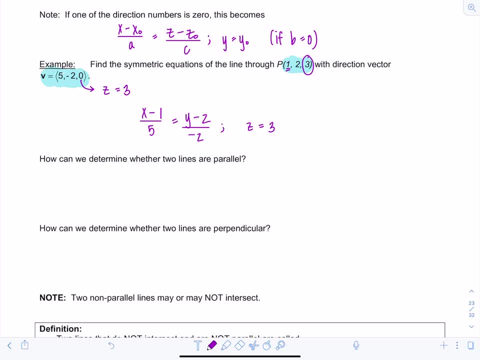 put a little semicolon, z is equal to three. All right, Nice. Now how could we determine whether two lines are parallel? What would you do? Well, it's pretty easy to look at the equation of the line, whether it's written parametrically or using symmetric equations, and determine what. 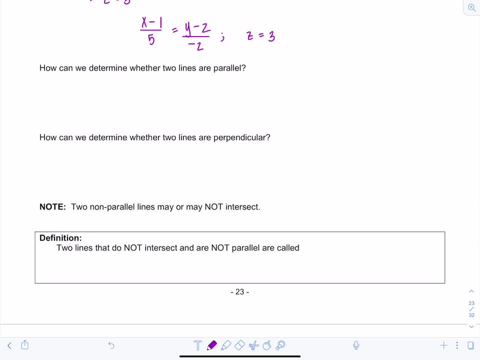 the direction vector is. So if you have the equations for two different lines, all you would need to do is check whether or not the direction vectors are scalar multiples of each other. If they are, then the direction vectors are parallel, which means the lines are parallel. 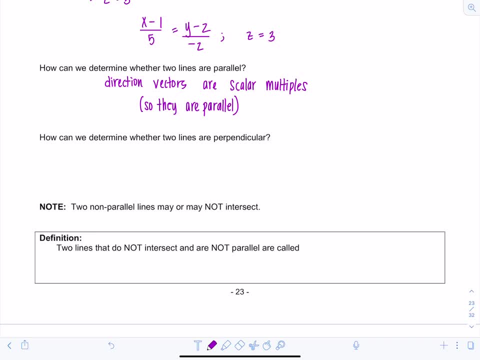 Now, similarly, how would you determine whether two lines are perpendicular? Well, if two lines are perpendicular, that means their direction vectors would need to be perpendicular. And how can you check if two vectors are perpendicular? Well, the best way to do that is by taking their dot product, So the dot product of the direction vectors. 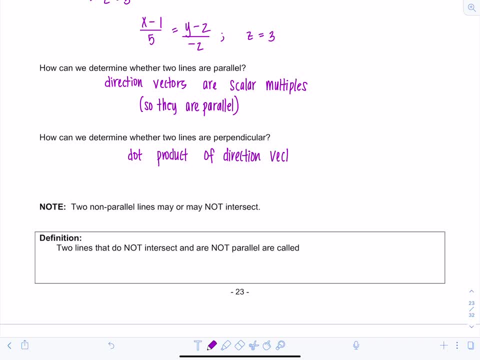 is zero. Okay, Now something interesting in free space that doesn't occur when you're just working in a plane- is that two non-parallel lines may or may not intersect, And the definition is: if you have two lines, they don't intersect. 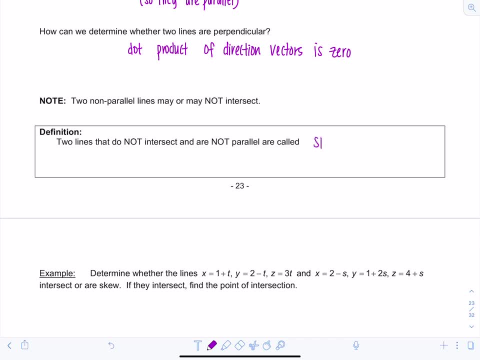 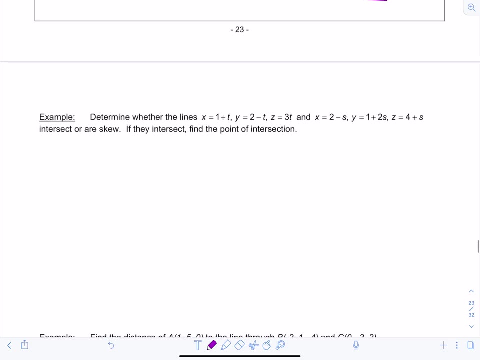 and they are not parallel. they are called skew lines. How is this possible? Well, basically, they live in different planes. Okay, So we're going to look at an example regarding how to determine whether or not this is the case. So, determine whether the 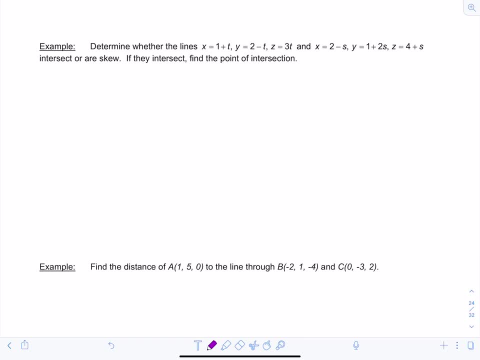 lines x equals 1 plus t, y equals 2, minus t, z equals 3t, So we'll call that line 1.. And the other line, x equals 1 plus t, y equals 2, minus t, z equals 3t, So we'll call that line 1.. 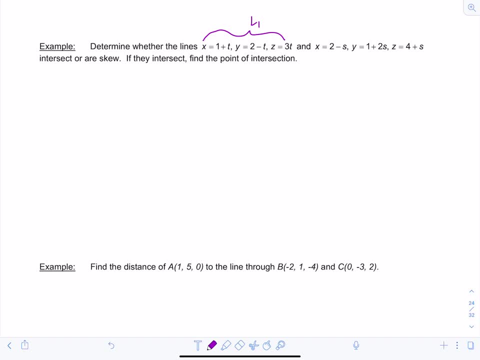 Y equals 1 plus 2s, z equals 4 plus s. We'll call that line 2. Determine whether they intersect or are skew And if they intersect, find the point of intersection. Okay, So the first thing I want: 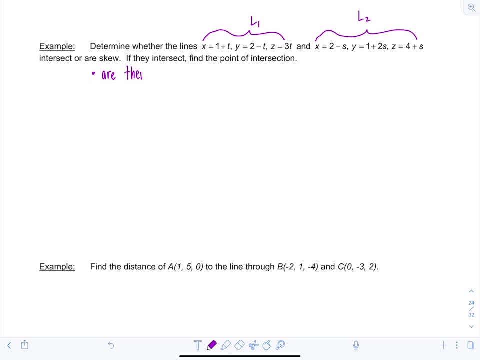 to ask is: are they parallel? Well, what's the direction vector for the first line, Can you tell You? just look at the coefficients on t. So the first component is going to be a 1. The next component is going to be a negative 1.. 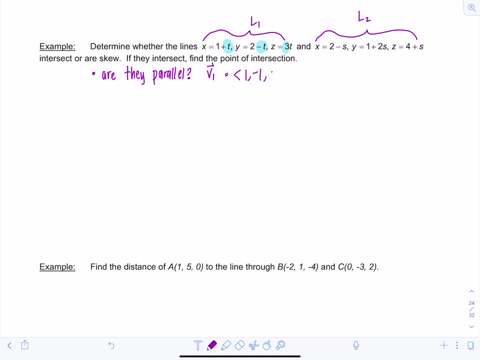 And then the last component is going to be a 3. So that's the direction vector for the first line. What's the direction vector for the second line? The components would be negative: 1,, 2,, 1.. Well, clearly I can see these are not scalar multiples, So I know the lines are not parallel. 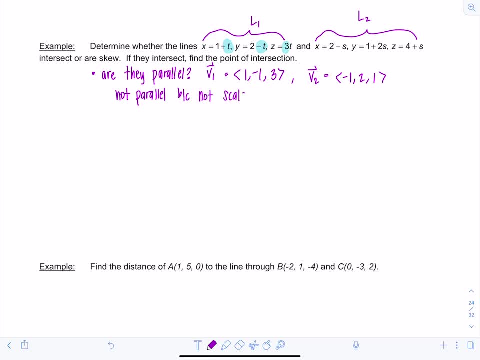 Because they're not scalar multiples. Okay, Now let's check if they intersect. How would you go about doing that? Well, what does it mean for two lines to intersect? It means that they share a point in common. It means that they would have to have an x, a y and a z coordinate in common. So if they have an x coordinate in common, that means 1 plus t needs to equal 2 minus s. Well, at the same time, they have to have a z coordinate in common. So if they have an x coordinate in common, that means 1 plus t needs to equal 2 minus s. Well, at the same time, they have to have a z coordinate in common. So if they have an x coordinate in common, that means 1 plus t needs to equal 2 minus s. 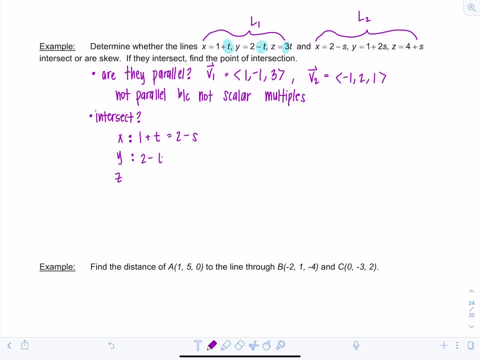 Well, at the same time they have to have a z coordinate in common. So if they have an x coordinate in common, that means 1 plus t needs to equal 2 minus s, 2 minus t would have to equal 1 plus 2s And lastly, 3t would have to equal 4 plus s. I have two unknowns. Can I simultaneously solve this system so that x, y and z all intersect? 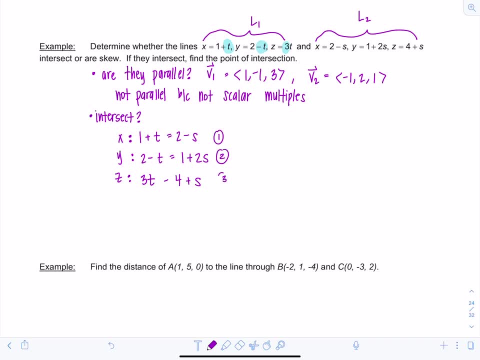 Let's number these equations: 1,, 2, 3.. I'm just going to focus on equations 1 and 2 for now, Okay, And solve that system. I have more equations than unknowns, so what I'm going to do is solve just two equations at a time. 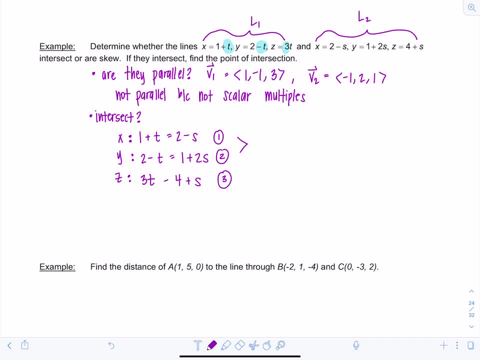 solve for those two variables and then substitute that solution into the remaining third equation. If it holds true, then I found a point of intersection. If it doesn't, then there's no solution to the system. So I can just add equations one and two together and notice. 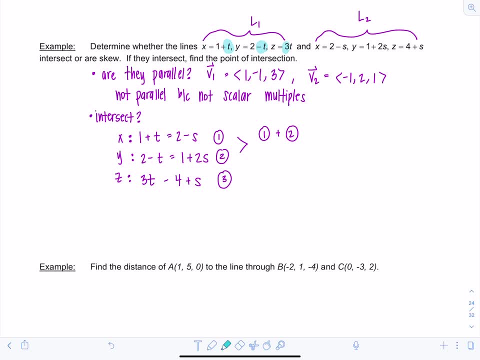 t is going to cancel out, right? So if I add these two together, add this and this, then that t is gone, right? So you're just going to have: three is equal to three plus s, which would mean s equals zero. And if s is equal to zero, you could just substitute in to whatever equation here, plug in. 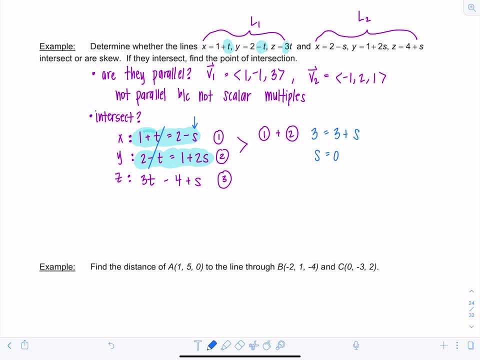 a zero there. for s subtract over a one, that means t is equal to one. Okay, I'm going to check this solution now of s equaling zero and t equals one into the equation that I didn't use. check it into equation three. So is three times one. is that equal to four plus zero? No, 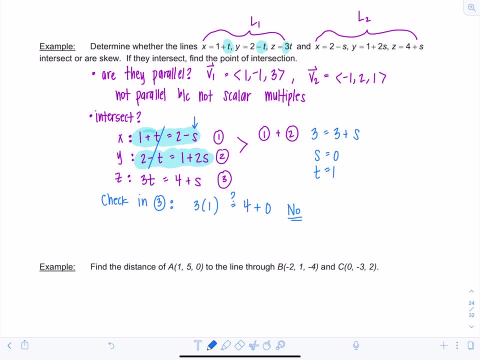 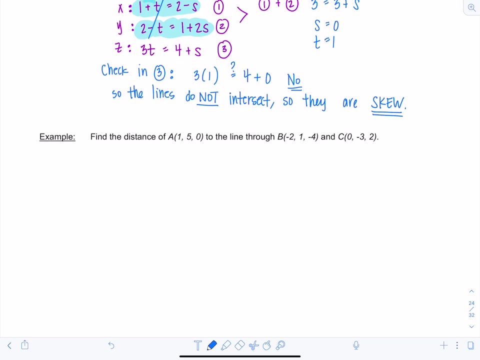 So that means there's no solution to the system, which means the lines do not intersect, So they are skew. Okay, very nice. Now let's look at an example of a question that's going to come up in several different contexts. So say, we want to find the distance from a point to the line that goes: 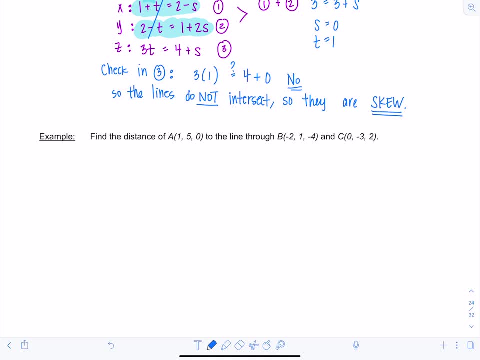 through two other points. I'm going to draw a picture. I know we're working in three-dimensional space, but I'm just going to draw it like we're in a plane to kind of help orient things. okay, So say we have a line. 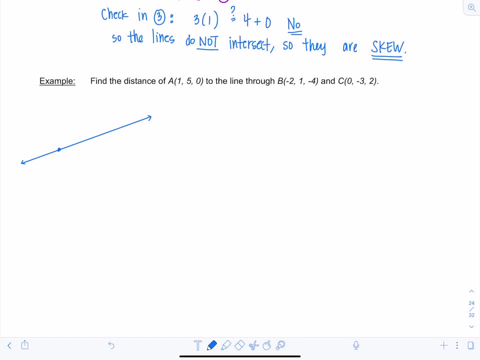 and it goes through the points b and c. So I'll put b here, I'll put c here and I want to find the distance that a is from that line. So whenever we talk about the distance from a point to a line, 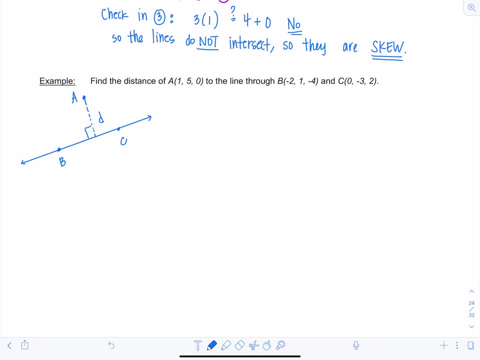 it's implied that we want the shortest distance, the one that intersects at a 90-degree angle that hits it at an altitude, okay. So what are your options here? We've got quite a few. First thing that we absolutely have to do is we're going to have to make a vector here from b to a, okay, And then I 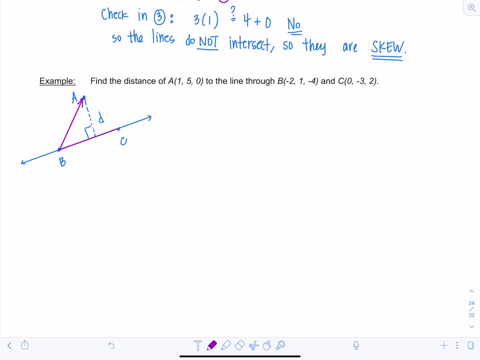 have another vector here connecting the two points b and c. okay, So one way that you could find that distance is by using Pythagorean theorem, Option one. So how would you do it using the Pythagorean theorem? Well, you're going to have 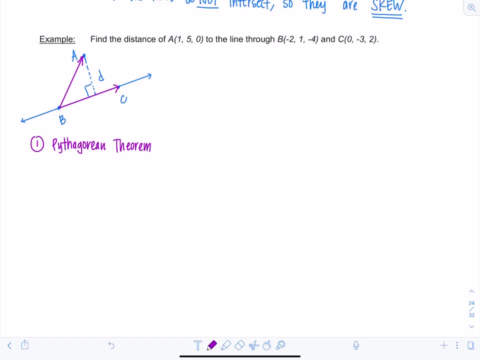 a squared plus b squared, and then you're going to have a squared plus b squared, and then you're going to have a squared plus b squared equals c squared. Well, a squared, or one of the sides squared. let me draw it out for you: this distance here, that's going to be the scalar projection. 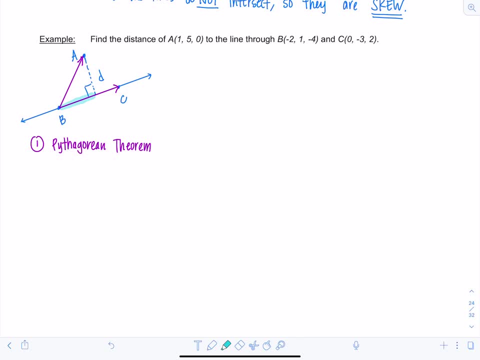 of vector b a along vector b c, right, Do you agree? So I'll write that in here. This is the scalar projection of vector b a along b c. So if I'm using the Pythagorean theorem, I'm going to. 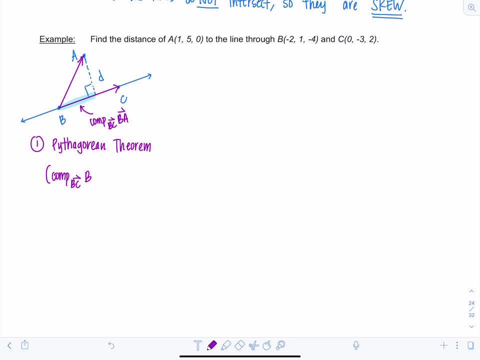 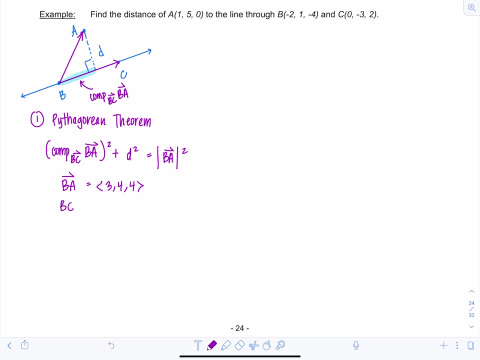 have that scalar projection squared plus the other leg. squared is equal to the hypotenuse, that would be the magnitude of b a squared. And then how would you in practice go about solving it? Well, you'd have to make your little vectors b a, which is 3,, 4, 4,, and then b c, which is 2, negative 4, 6.. And then you can go ahead and use the 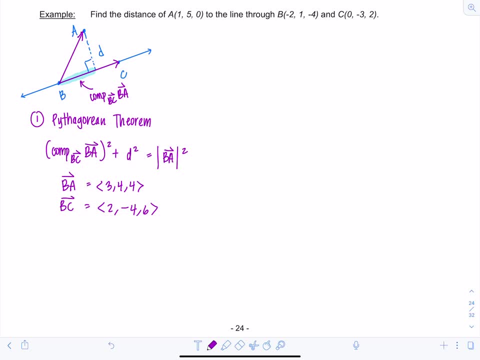 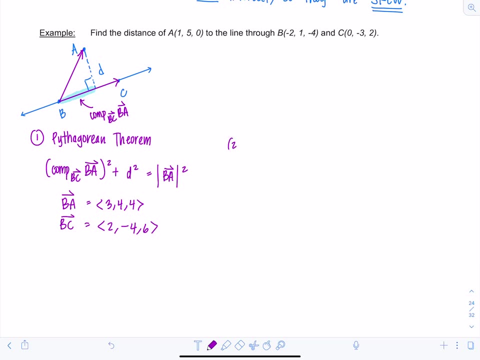 definition of your scalar projection. find the magnitude of b a squared, and then you just solve for the distance squared. There's option one. Option two, d, is the absolute value of the orthogonal projection of b a along b c. So you could solve it that way And remember. 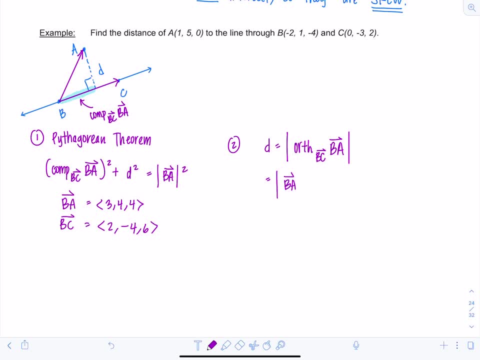 our orthogonal projection is b a minus the vector projection of b a along b c. Okay, and since I want it to be distance, I'm going to take absolute value. Last way would be using trig, but we're going to end up not needing the angle, So I'm going to set. 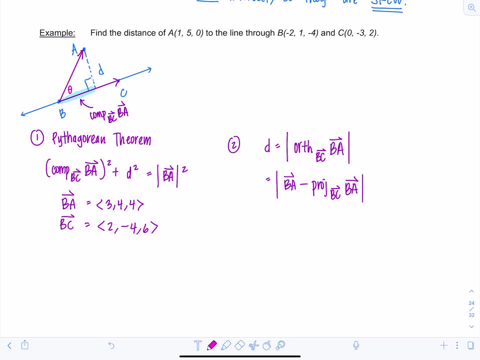 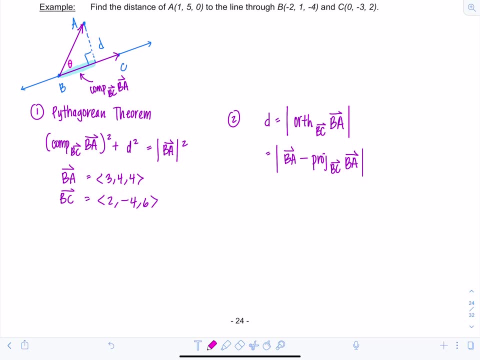 it up where I'm going to involve the angle theta. but notice it wasn't given, So I'll show you how. you don't actually need it. So what we're going to do is express the ratio of d with one of the other sides here that we can compute. So we're going to do that, And then we're going to do: 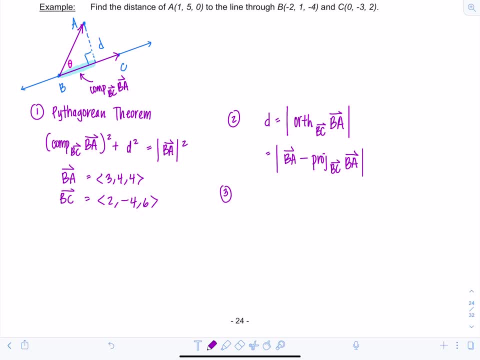 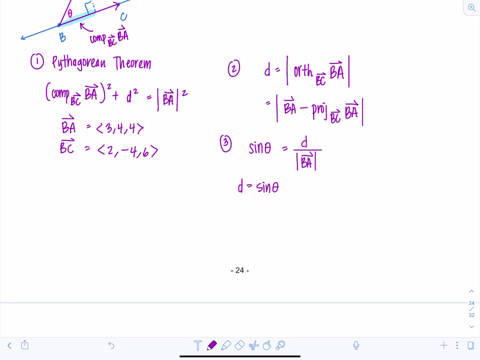 that. So I could write option three, that sine of theta is equal to the distance divided by hypotenuse, which would be magnitude of b a. So that means the distance is equal to sine of theta times the magnitude of b a. But remember, we have that nifty property of the cross product. 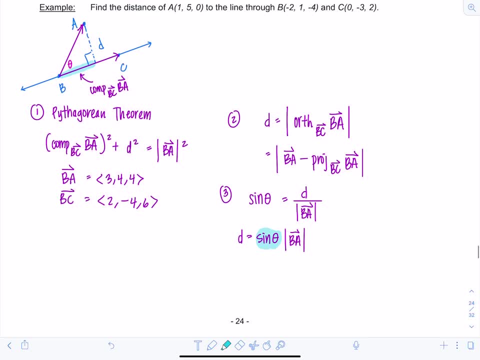 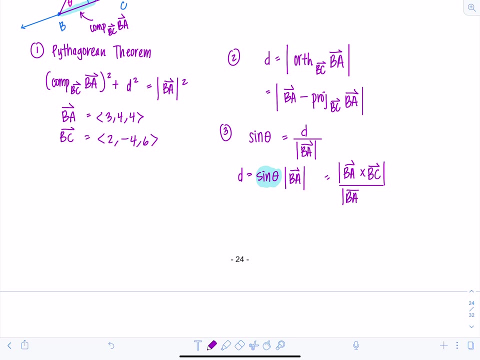 which tells me that sine of theta is equal to the magnitude of b a crossed with b c, divided by the magnitude of each of those vectors. So the magnitude of b a times the magnitude of b c. So what's highlighted is equivalent. This is equivalent to sine theta. That's from the lesson on the cross product. 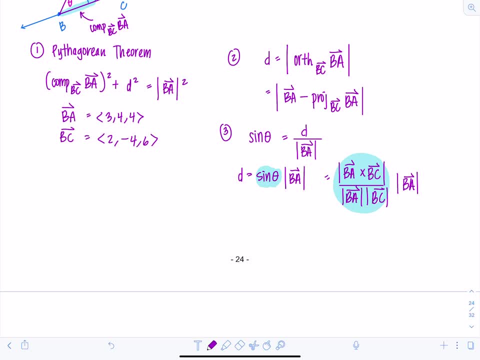 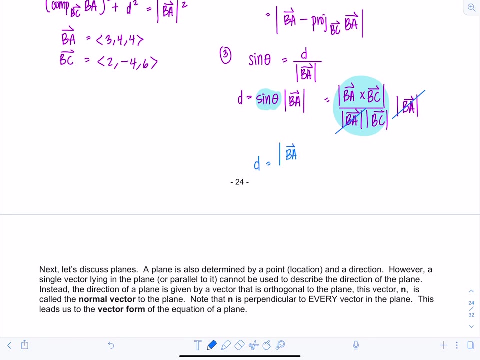 And then I still have times. magnitude of b a, And then notice I can cancel out magnitude of b a And then you're just left with the distance is equal to magnitude of the cross product b a and b c divided by magnitude of b c. 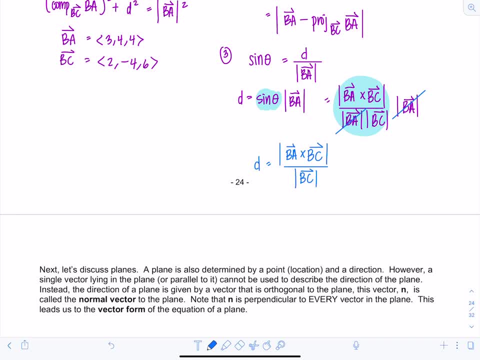 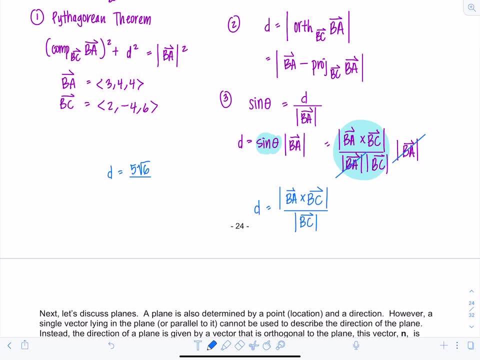 So I'll leave it up to you. Actually, you should verify that you can solve it all three ways and find the distance, And to verify that you did it correctly, you should get five rad six over two, But I'll leave it as a matter of fact. So I'll leave it as a matter of fact. 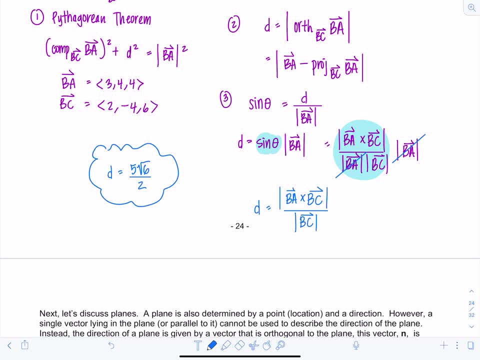 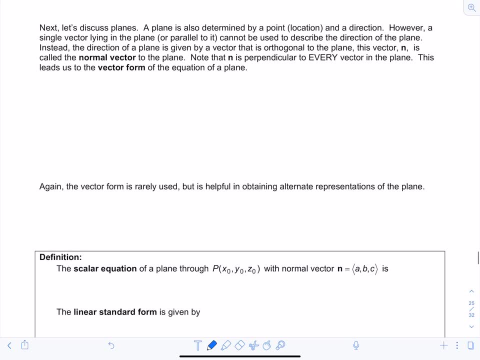 exercise for you to do. Okay, that concludes our discussion of lines for now. Now we're going to discuss planes, And a plane is also determined by a point, which is a location and a direction. However, if you just have a single vector lying in the plane, or a vector that you say is parallel, 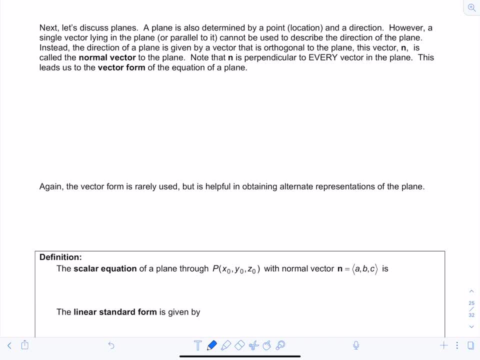 to the plane. that's not enough to describe the direction of the plane. There's infinitely many possibilities if you just give a vector that's parallel to the direction of the plane. Instead, if you want to uniquely describe a plane, its direction, you need a vector that's orthogonal. 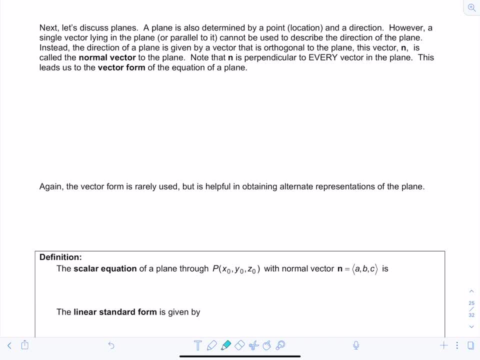 to the plane And we call this vector n, the normal vector. Okay, Now notice that n is going to be perpendicular to every single vector that's in the plane, And this leads us to the vector form of the equation of the plane. So I'll draw you a little picture here. So when you're writing the 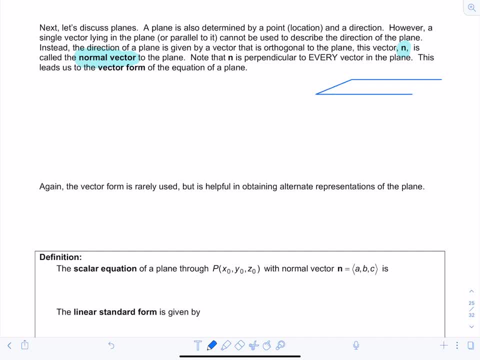 equation of a plane. okay, all you need is some point p And then you need a vector that is normal to the plane. Here's n, my normal vector. Okay, Now I'm going to let let's call this p-naught actually. So let's let p-naught have coordinates. 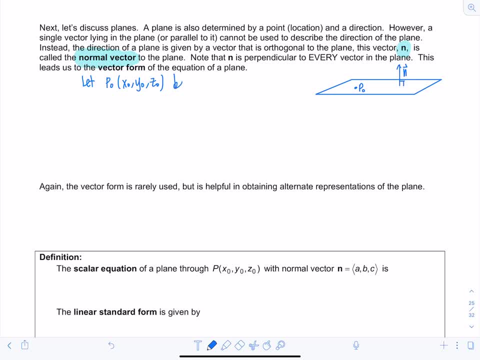 x-naught, y-naught, z-naught. That's going to be a fixed point on the plane. Okay, And I'm going to say p with coordinates x, y, z, y, z is an arbitrary point in the plane. Any other point that's in the plane. 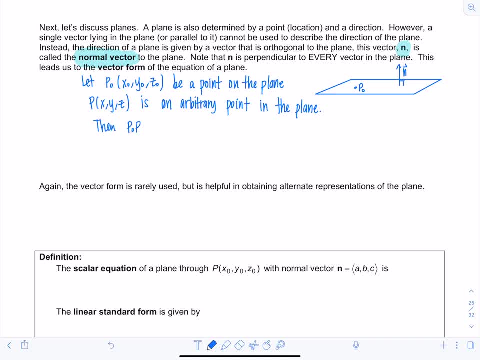 Then the vector p-naught, p is a vector in the plane. So imagine p is any other point in the plane, right, Say it's over here, You can draw it anywhere you want. So P, not P. if I make that vector, that's going to be a vector in the plane. 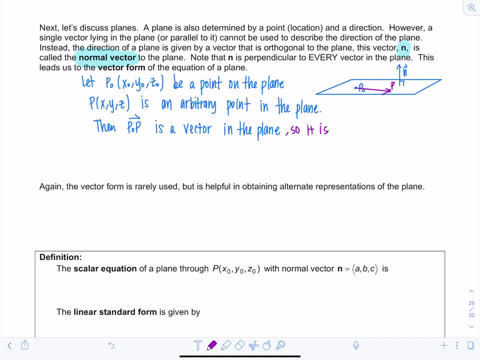 What does that mean? So it is perpendicular to the vector N, the normal vector. Well, what do I know is true about vectors that are perpendicular? I know that their dot product is going to equal zero, which means N dotted with, and we saw on the previous notation for writing equations of lines. 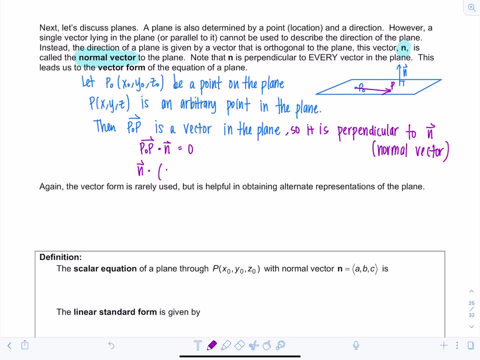 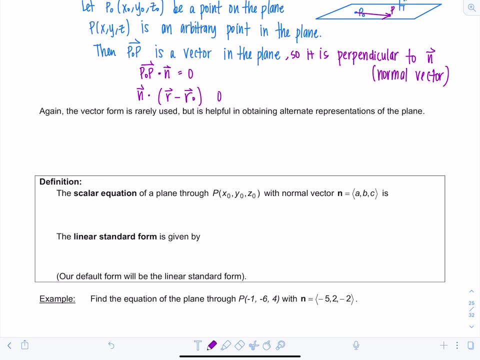 we're going to introduce that again here, For P, not P. you could write it as R minus R, not equals zero. Okay, so the vector form is rarely used, But it's helpful in obtaining an alternate representation of the plane. So say, your normal vector has components A, B, C. 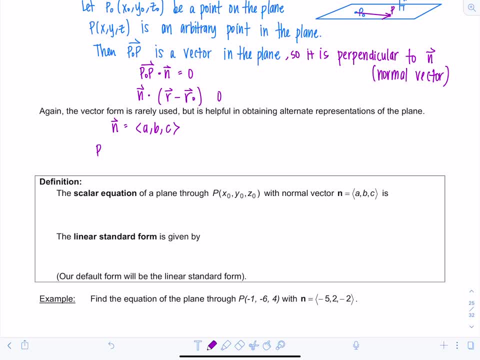 Okay, and you want to make your vector P not P right. P not P. Well, it would have components X minus X, not Y minus Y not and Z minus Z- not right, Since P's coordinates are X, Y, Z, P not's coordinates are X not Y, not Z not. 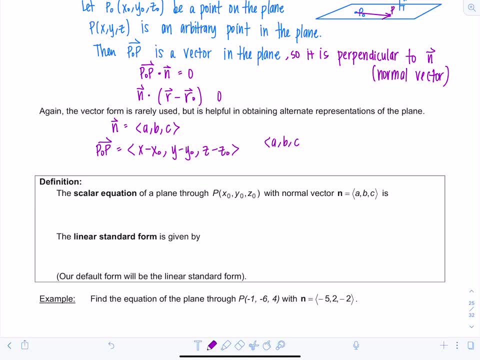 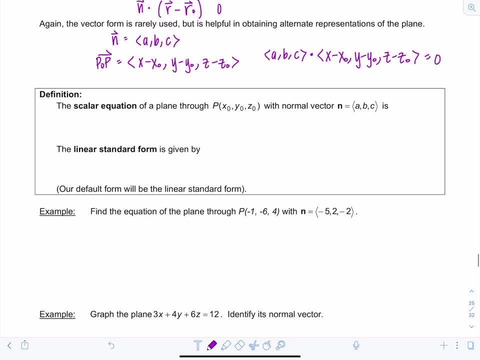 And then the equation would be A, B, C, Dotted with X minus X, not, Y minus Y, not Z minus Z. not is equal to zero. Is that how we actually write the equation of a plane? No, What we do is we take the dot product. 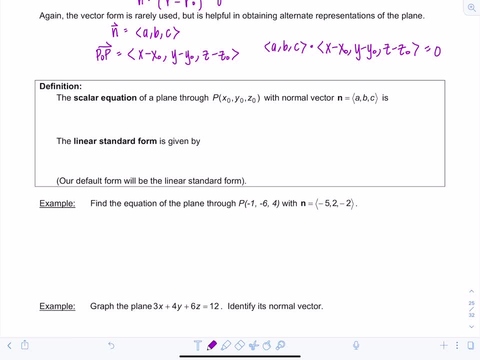 So the scalar equation of the plane is given by the following: We have A times X minus X, not plus B. times Y minus Y, not plus C. times Z minus Z, not is equal to zero. That's the scalar equation And the linear standard form is given by: AX plus BY plus CZ equals D. 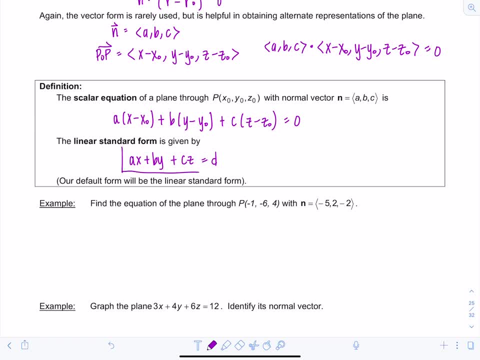 where you clean up and move all the constants to the other side. Now, this is the form that's required for class. okay, If I'm not your instructor, check with them what they want. Okay, So let's look at some examples. 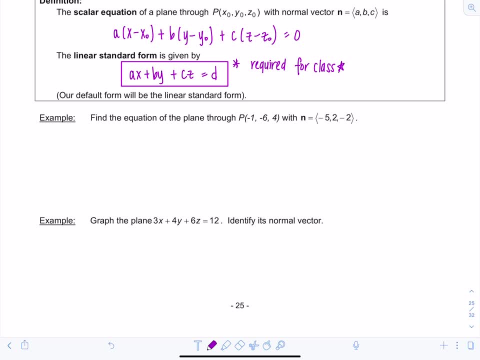 So let's look at some examples here. Find the equation of the plane that goes through point P with normal vector given there, So you can just jump straight to the scalar equation and then clean up so you get linear standard form. So what do I mean by that? 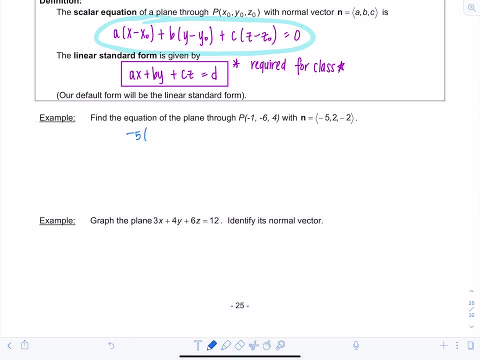 So I'm going to write this as negative 5 times X minus negative 1,. so X plus 1, plus 2 times I'm going to have Y plus 6, minus 2 times Z minus 4, is equal to zero. 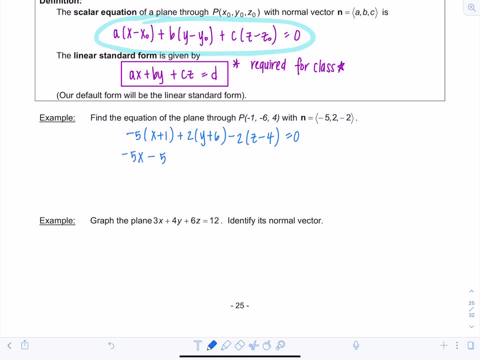 And then we're going to clean up here. So we have negative 5X minus 5 plus 2Y plus 12, minus 2Z plus 8 is zero, And so I end up with negative 5X plus 2Y minus 2Z is equal to negative 15.. 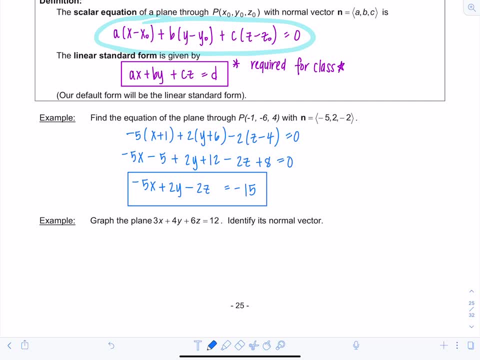 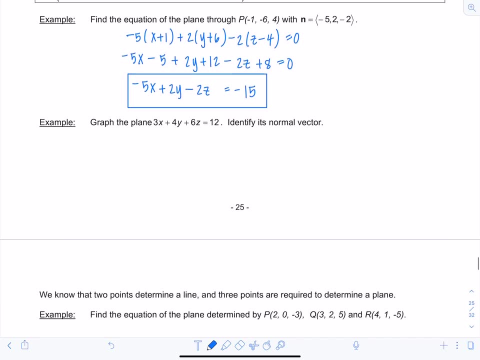 Okay, Good, That was a pretty straightforward example. Now we're going to graph the plane 3X plus 4Y plus 6.. Z equals 12, and identify its normal vector. Well, the normal vector I can spot right off the bat by just. 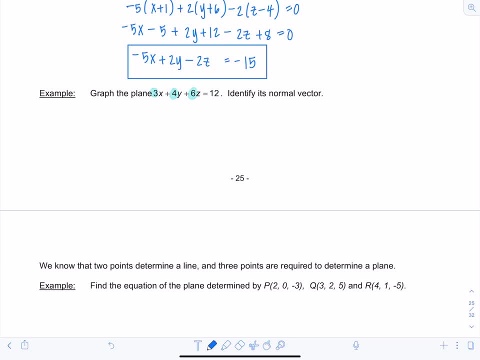 taking those coefficients off of each of the variables there. So the normal vector, I know, has components 3,, 4, 6.. Okay, And then to graph it, what we're going to do is graph each of the traces. So what do I mean by that? 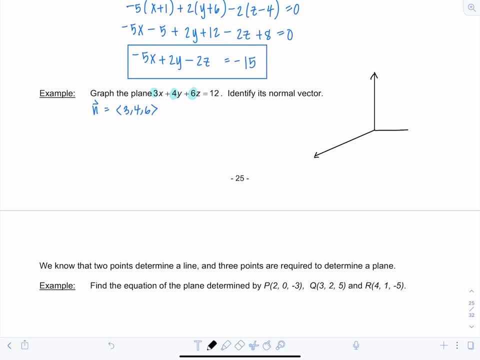 What we're going to do is set a different variable equal to zero, one at a time, and graph the trace in each of the planes. So here's X, Y, Z axes. Say, I'm going to graph the XY trace. Well, that would be from when I set Z equal to zero. 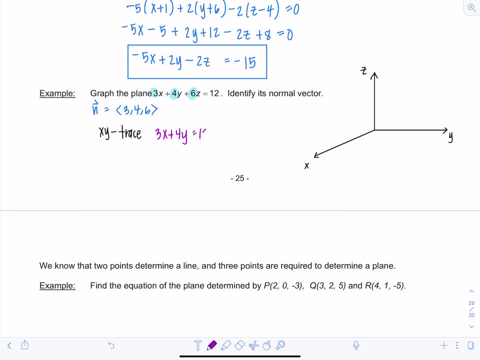 So that would give me the line 3X plus 4Y equals 12.. So I'm just going to graph that in the XY plane I can see that it would have an X intercept of 4 and a Y intercept of 3.. 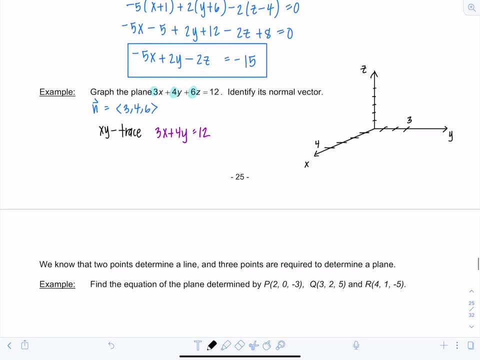 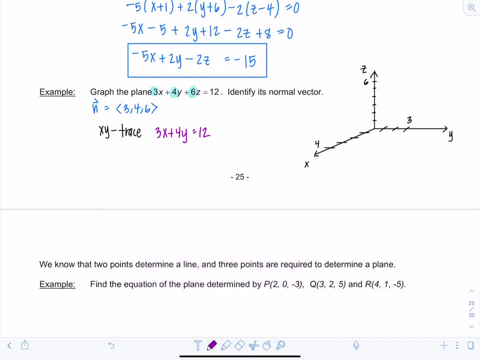 1,, 2,, 3,, 4,, 5,, 6.. So I'm going to graph that. So I'm going to graph that line. the XY trace, 3X plus 4Y equals 12.. Okay. 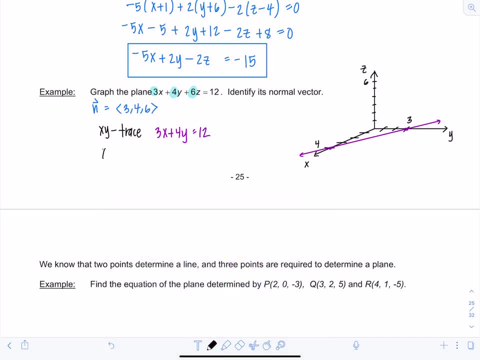 And then let's do another trace. So I'll do the XZ trace. So that comes from setting Y equal to zero. So then I'd have 3X plus 6Z equals 12.. Again, each of the intercepts there I'd have 4, 0, 0.. 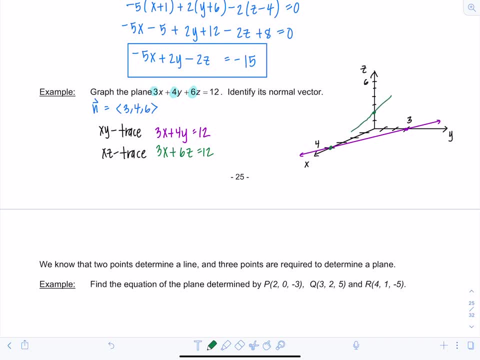 And then 0, 0. So I'd have this line in the XZ plane. And then, lastly, I could draw the YZ trace, And we'll do that in pink. So I will have: 4Y plus 6Z is equal to 12.. 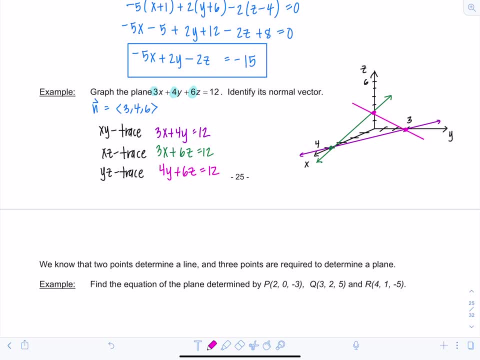 So I'm just going to connect these two points here. Okay, I'll list out what each of these intercepts are. So we have 4, 0, 0, 0, 3, 0, and 0, 0, 2.. 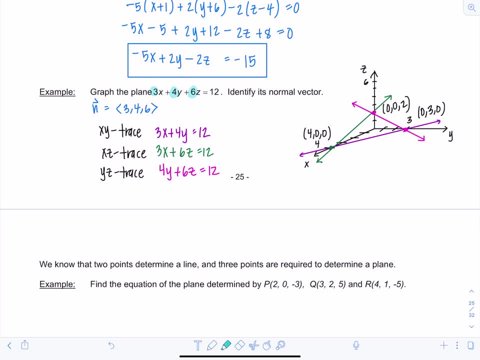 Okay, And if I just want to shade in, maybe the portion of the plane that lies within the first octant, it would be this little triangular region here, But remember the plane extends forever. So that triangle just represents the portion of the plane that's in the first octant. 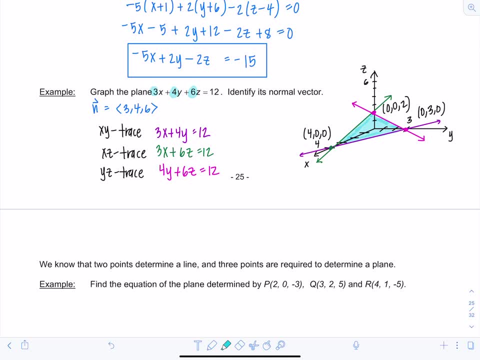 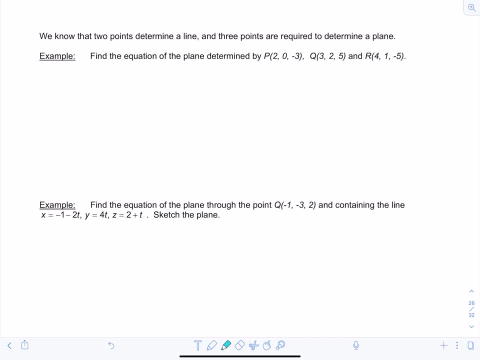 Okay, Good, Good, Now let's move on. We're going to do some further applications. Now we know that two points are needed to determine a line uniquely right, And similarly, three points are required to uniquely determine a plane. So we're going to find the equation of the plane determined by the points P, Q and R. 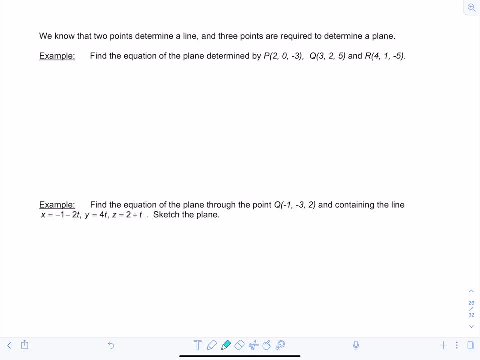 And let's think about how we would do that. So I know for sure I need a point that's in the plane. Okay, No problem, I got three of them. Okay, I have more than what I need. The other thing that I need is a normal vector. 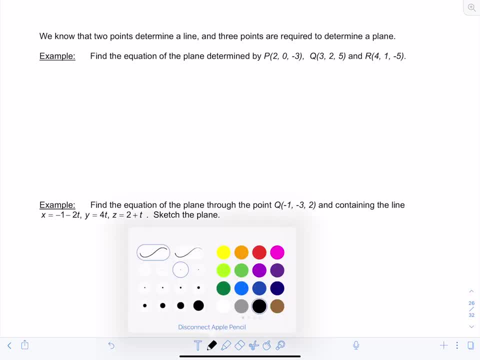 Normal to the plane. If I have three of them, I have more than what I need. So if I have three points that lie in the plane, how could I get a vector that's normal to the plane? So let's see here. 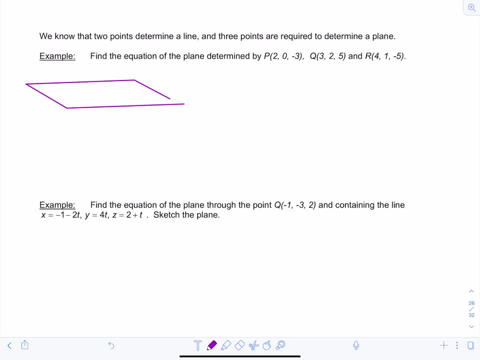 Let's draw a little picture, See if it's illuminating. Okay, So here's point P, Here's point Q, Here's point R. I want a vector normal to the plane. Well, what if I make a vector P, Q? 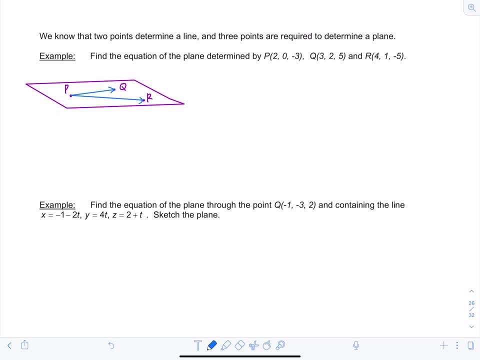 What if I make another vector, P R? Is there something special I could do with those vectors so that I get a normal vector to the plane? Why, yes? Maybe you're thinking, take their cross product, And that's precisely what we're going to do. 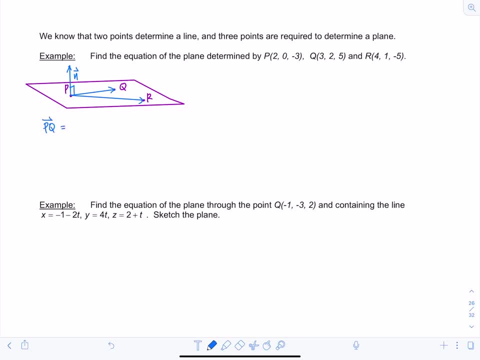 Okay, So the vector P, Q, Remember you take Q minus P, final minus initial, So that would have components 1,, 2,, 8.. And you know what? It doesn't matter if you make P, Q or Q, P. 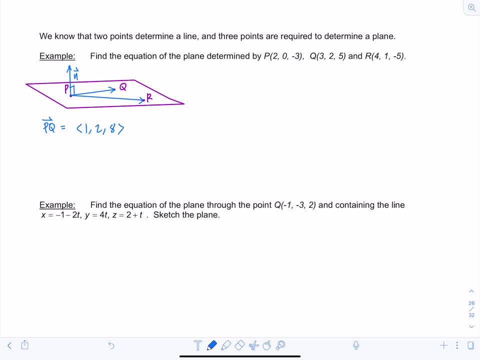 Just be consistent in how you create the vectors, that you use the same initial plane. So we have P Q, Then we have P R. P R has components 2, 1, negative 2.. And then now I'm going to take the normal vector. 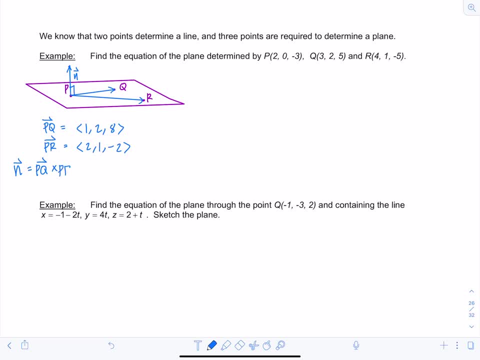 I'm going to find it by taking their cross product, So P Q crossed with P R. Are you getting good at doing this mentally? So you're going to imagine crossing this out, crossing out the I, J, hat, K, hat. 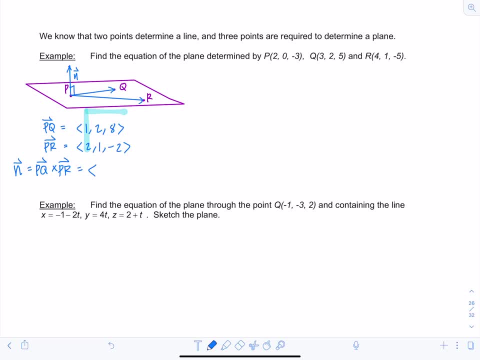 So you're going to have negative 4 minus 8. So that's negative 12.. Then the next component would be 16 minus negative 2. So that's 18.. And then, lastly, you would have 1 minus 4.. 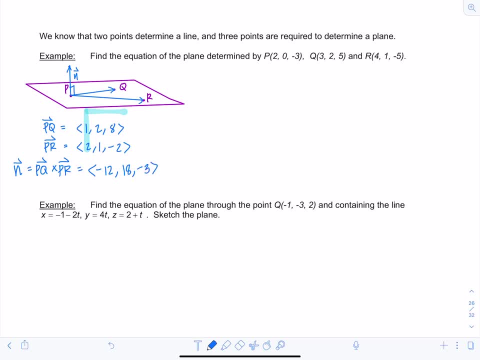 So negative 3.. Now I could go ahead and use this vector. That's fine, But notice, I could divide out a 3.. And it would look even better if I divided out a negative 3. That way, the first component would be positive. 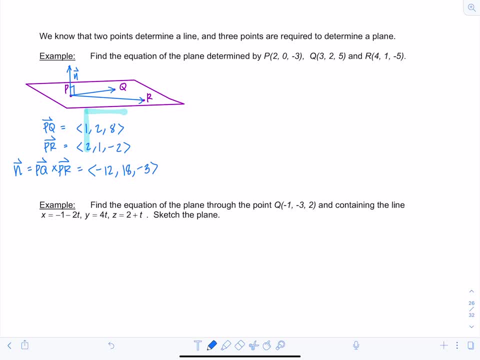 And that's just to make our equation more manageable, more user-friendly and more visually appealing. So what we're going to do instead is let's use 4, negative 6, 1 for N, And remember, any scalar multiple of that cross product is still going to be normal to the plane. 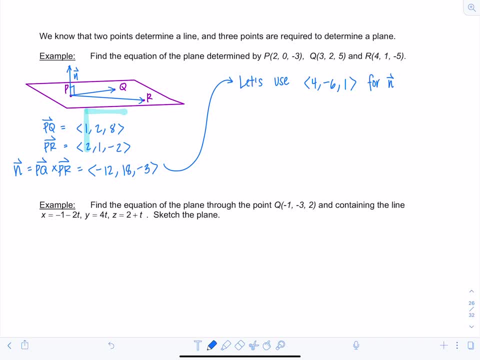 It's just going to be a little bit nicer of a vector to work with And then you can use any point as your P knot. So let's just use the first point P here that they gave us, But any point will work. That's on the plane. 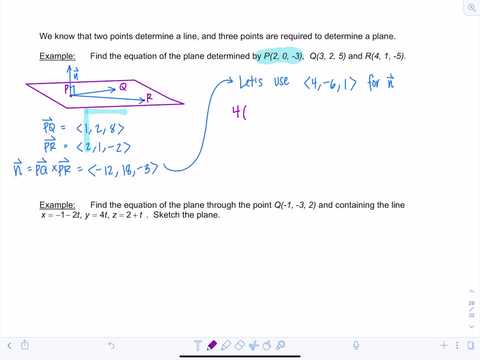 So we'll have 4 times x minus 2 minus 6 times y minus 0 plus 1 times z plus 3 is 0.. And then we want to go ahead and clean it up. So I'm going to have 4x minus 8 minus 6y plus z plus 3 is 0.. 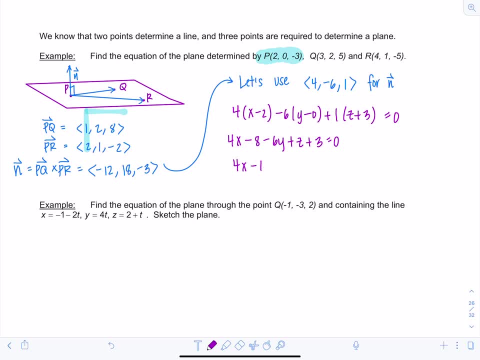 And then move all your constants to the other side. So we have 4x minus 6y, plus z is equal to 5.. OK, And you can verify. You'll get the same result if you went about it a different way, but followed everything correctly. 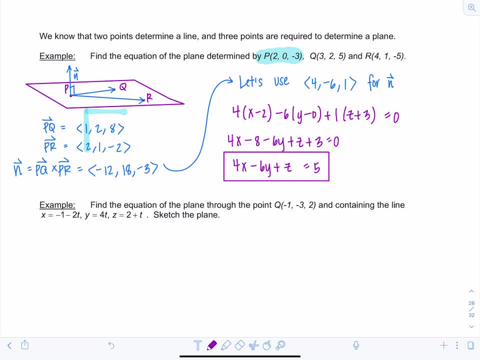 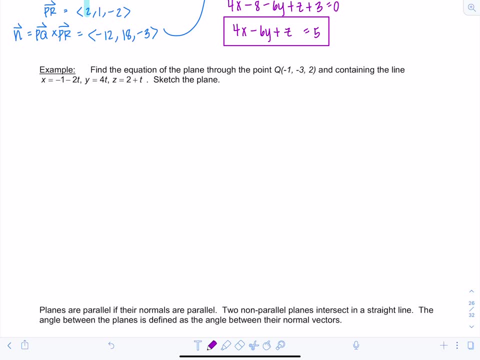 OK, Good. Next example: find the equation of the plane that goes through the point Q with coordinates negative 1, negative 3, 2, and that contains the following line: OK, So let's think about what's going on. So we have some plane. 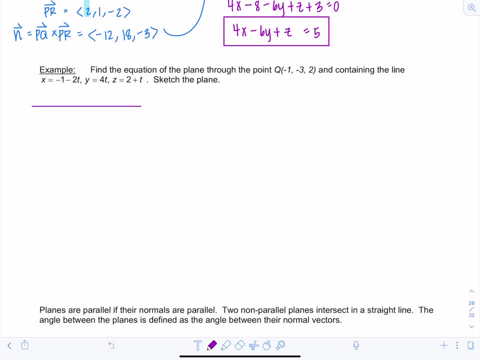 Here is my generic plane that I use for all examples. OK, We have some plane here And they're giving me a point, that's on it. And then also I've got some line in the plane. OK, Well, just think back. 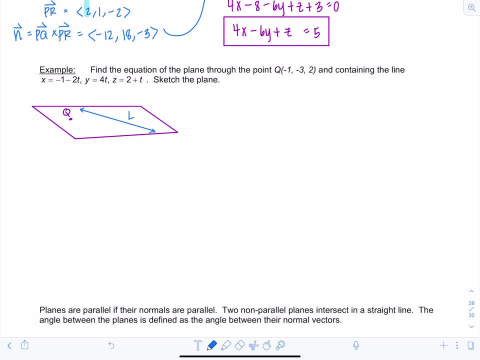 What worked before, when we were in a similar situation, when I had three points. Well, I took two vectors And I crossed them so I could get a vector normal to the plane. Well, I want to do something similar. I know that the line is in the plane. 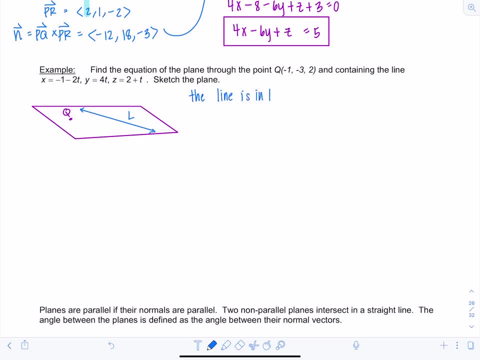 Right, That's given. So it's direction vector, the direction vector of the line v. Do you know what it is? Can you tell by looking? Do you remember You take the coefficients on t from the parametric equations. The direction vector has components negative: 2, 4, 1.. 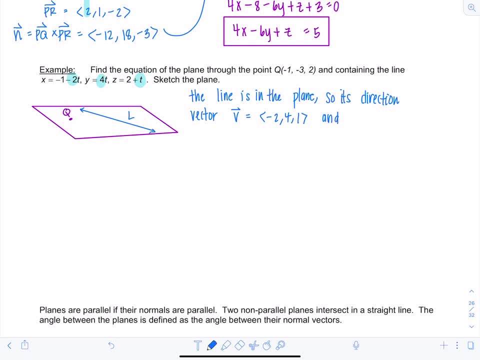 That direction vector and the point p. The point p has coordinates negative, 1,, 0,, 2.. You might be like: where in the world is that coming from? That's coming from plugging in t equals 0 into the parametric equations. 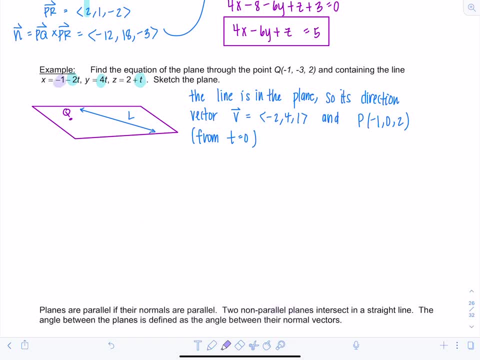 So notice, if I plug in: t equals 0, x is going to be negative 1, y is going to be 0, z is going to be 2.. So I know that point p, I know that point p is on the line and it's in the plane. 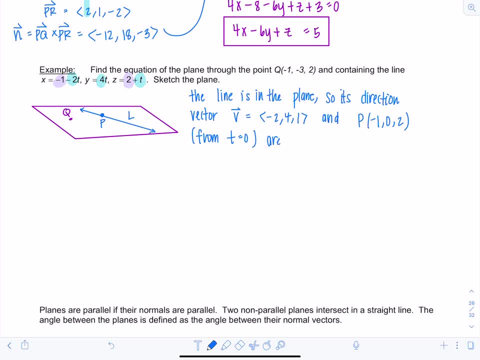 Okay, So both that direction vector and that point are in the plane. What to do now? I'm going to connect p and q. Why am I doing that? Because I'm going to try to be in a scenario, like I was in the previous problem, where I have two vectors that are in the plane. 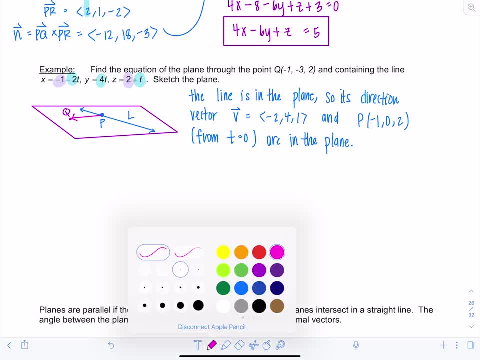 So I'm going to connect p and q, So I'm going to make vector pq. now, What are the components for vector pq? Well, here's p, Here's q, Let's make a vector. The components are going to be 0, negative, 3, 0. 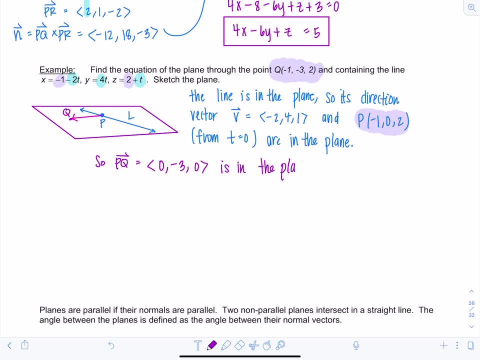 That is also in the plane. So, do you see, now I have two vectors that are in the plane. I have vector v, my direction vector, on the line. Now I don't know exactly how long it is or where it's going. 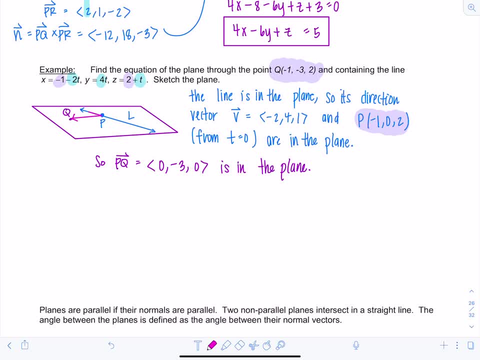 I don't even know how long it is, But the direction vector v, it's somewhere here. Okay, There's a vector in the plane. pq is also in the plane. How do I get a normal vector to the plane? That's right. 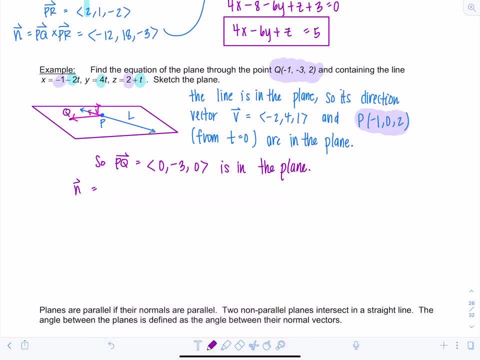 You take their cross product, So n is going to come from taking v crossed with pq. Okay, And let's go ahead. Let's do that, maybe off to the side here. So you have negative 2,, 4,, 1.. 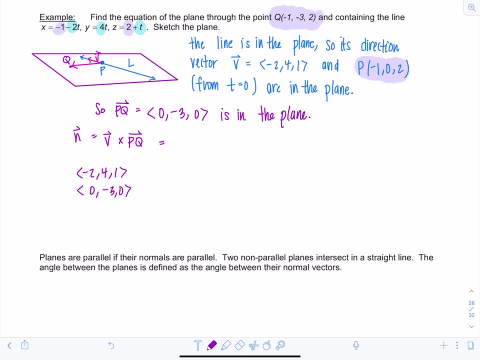 pq has components 0, negative 3, 0.. So this is going to be- imagine crossing this out. That would be 0 minus negative 3. So that's 3.. Next we're going to have cross this out, this out. 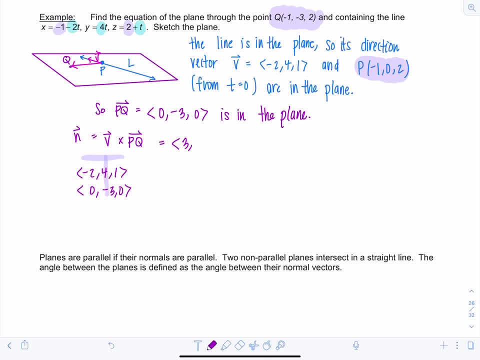 You do 0 minus 0. So the next component is 0. And then, lastly, we're going to have positive 6 minus 0. So this is 6.. Okay, So we could use 3,, 0,, 6.. 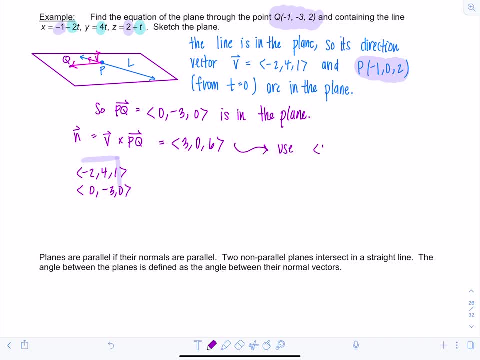 What would be nicer, though, is if we we use 1,, 0,, 2.. Okay, And then what point do we want to use? I mean, they gave us point q in the plane. You could also use point p. 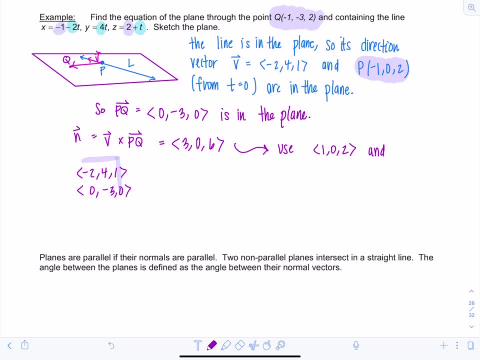 We know it's in the plane, But I'm just going to use q And q negative 1, negative 3, 2.. And let's go ahead and write the equation. So I'm going to have 1,, this 1, times x plus 1,. 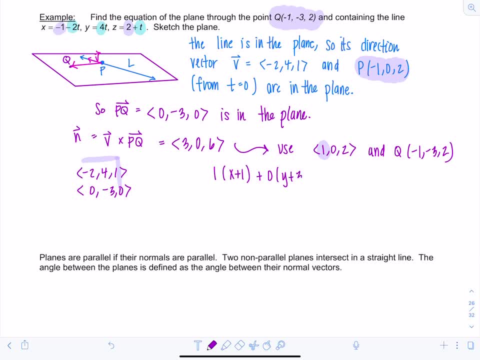 plus 0 times y plus 3, plus 2 times z minus 2 is equal to 0.. Ooh, okay, So this whole term's gone, So I'm just left with now. x plus 2z is equal to positive 3.. 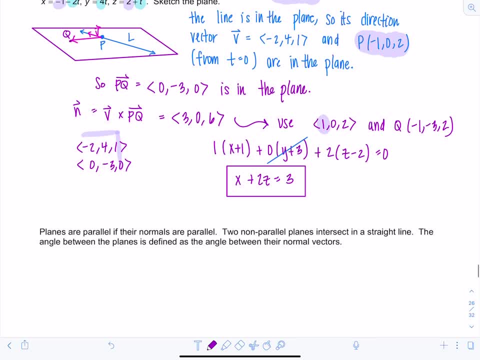 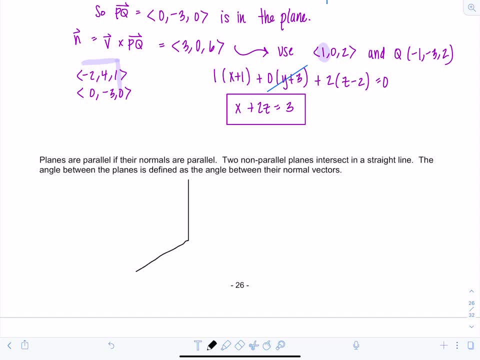 Okay, And then it asks us to sketch the plane. So you know what. I'll do that down below here. So there's my z-axis, X-axis, Y-axis, And if you just want like a nice, quick and easy way to sketch it. 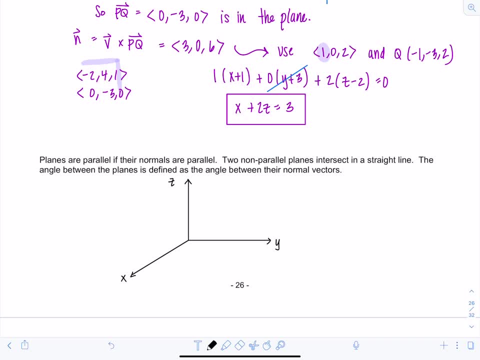 you can just write out: well, I know, x plus 2z is 3, so let's just get the intercepts. So I know, if z is 0,, y is always 0, right, So we're going to have 3, 0, 0 as a point on the plane. 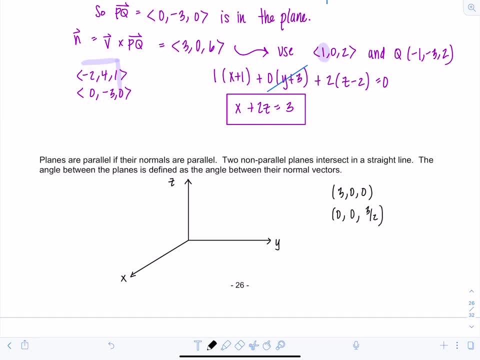 as well as 0, 0,, 3 halves. Okay, 1, 2, 3.. 1, 2, 3.. And then y is always 0.. So we're going to go through 3, 0, 0.. 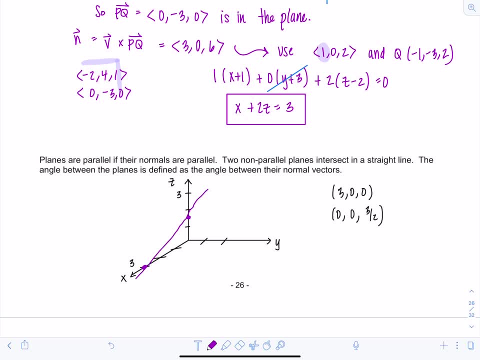 0, 0, 3 halves. So I have this line in the xz plane. I'm not happy with that. Bear with, Let's see if this is better. Okay, I have this line in the xz plane. 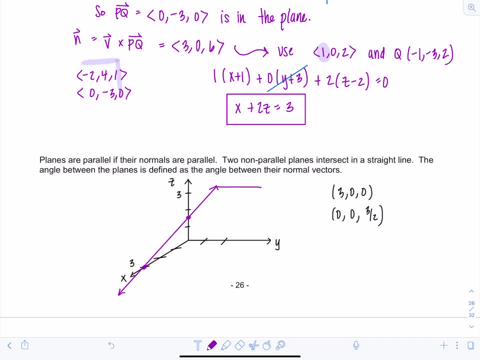 And then y is equal to 0. So I'm going to be extending out this way, Okay, And I'm drawing it, you know, as sort of a rectangle, But remember it extends forever. All right, Good. Now returning to the lesson. keep in mind: planes are parallel. 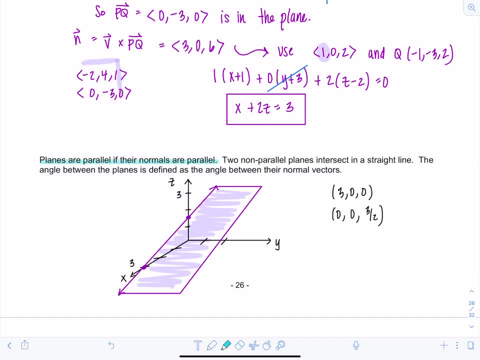 if their normal vectors are parallel And two non-parallel planes intersect in a straight line. You could imagine if you have two planes, they're not parallel and they intersect. their intersection is going to be an entire line And the angle between the planes is defined as the angle between their normal vectors. 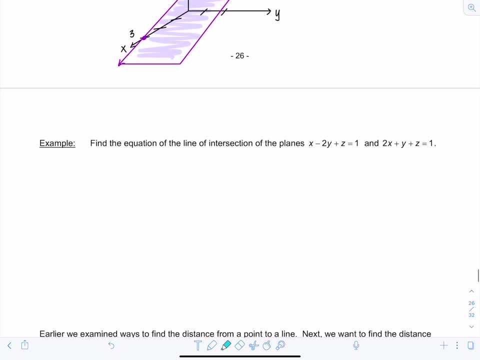 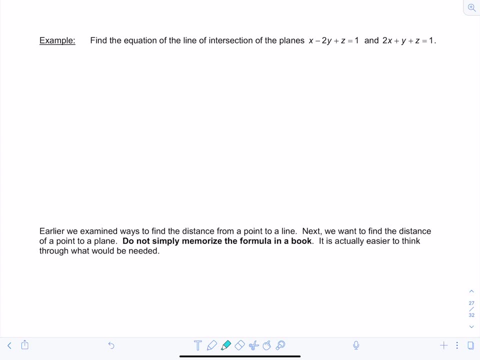 So let's look at how to apply this: Find the equation of the line of intersection of these two planes that are given here. Okay, So how would I find the equation of the line of intersection? Well, think first. what do you need to write the equation of a line? 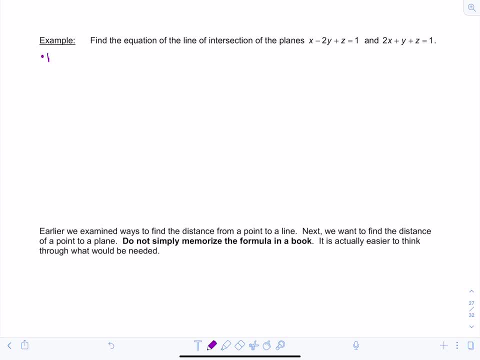 You need a point that's on the line, And then you also need the direction vector. Okay, And think about it this way. So we've got two planes and they're going to intersect and their intersection is a line. So here's plane number one. 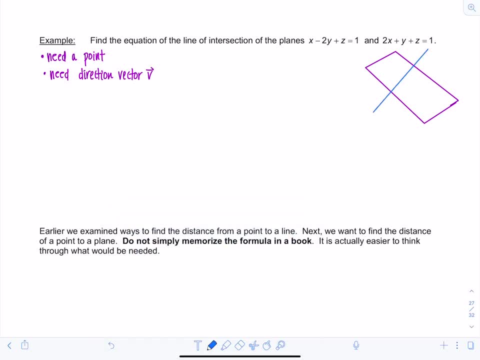 And then let's draw plane number two, Okay, And they're going to intersect and their intersection is a line. Okay, Now, each of these planes, we know what their normal vectors are, right? So there's a normal vector for one plane and then there's a normal vector for the other plane. 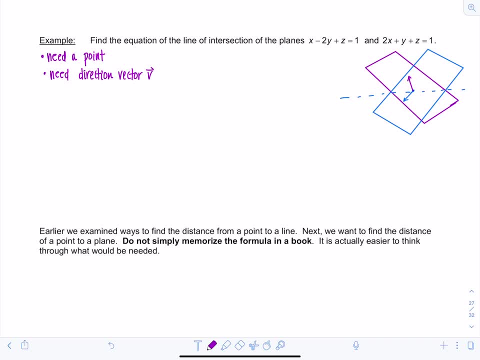 Okay, So let's see, Can we figure out a point that is in both planes? Well, by observation I can see that the point is in both planes. Okay, That's just by observation. If you can't easily observe, then you just solve. 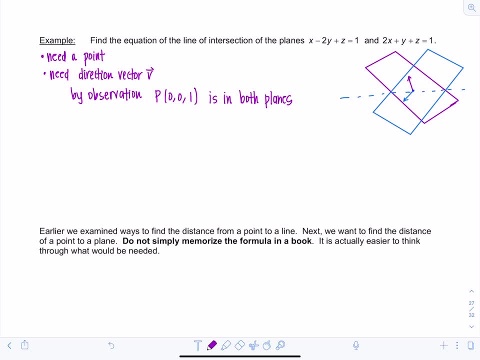 You plug in something for x, you plug in something for y, and then you solve and find a point that's on both lines. Okay, Well, no, Just plug in something for one variable and then solve for the other two, so you find a point that's on both lines. 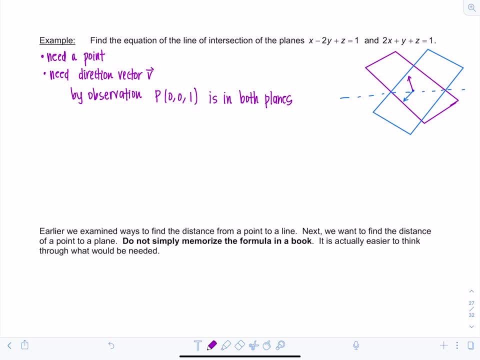 Okay, In this case I lucked out, I didn't have to do that. So that means that point P it is on the line of intersection. What else is on the line of intersection? Well, before I get there, I want to think about this actual line of intersection. 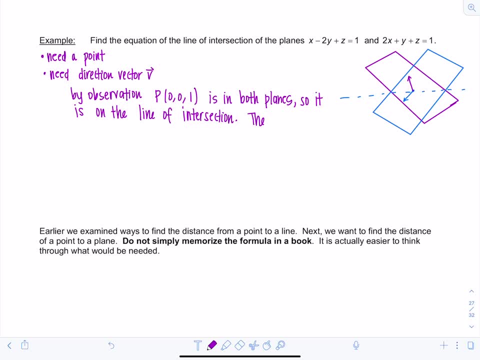 This line lies in both planes, So it's perpendicular to both of their normals. What are the normal vectors for each of the lines? Well, normal vector for line number one. I'm just going to look at the coefficients here on the variables. 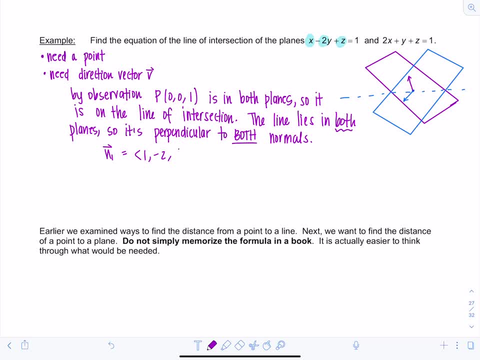 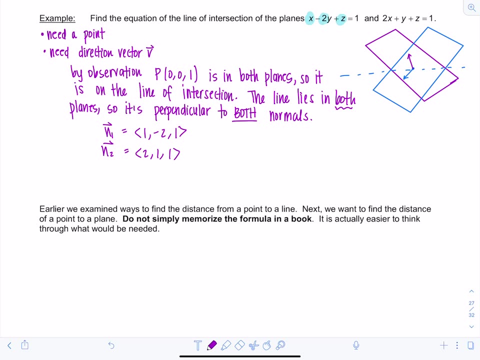 So the normal vector would be 1, negative 2, 1.. And then normal vector number two would be 2, 1, 1.. So if my direction vector for my line is perpendicular to both normals, then that means I could find it by taking the cross product of those two normals. 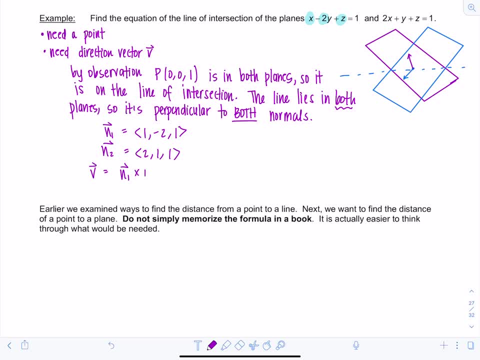 So the direction vector can be found by taking n1, crossed with n2, which would give me negative 3, 1, 5.. All right, So that means I have a point, I have the direction vector. Now I can write the parametric equations of the line. 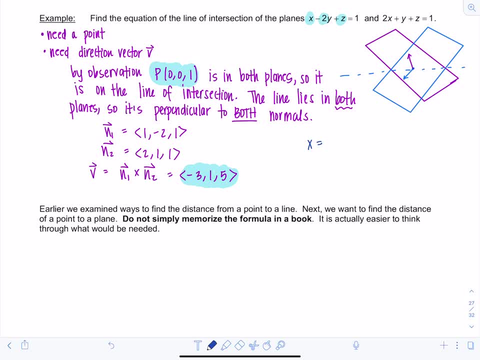 So the line would have: x equals 0 minus 3t, So just negative 3t, y would equal 0 plus 1t And z would equal 1 plus 1t. So that's our final answer, All right. 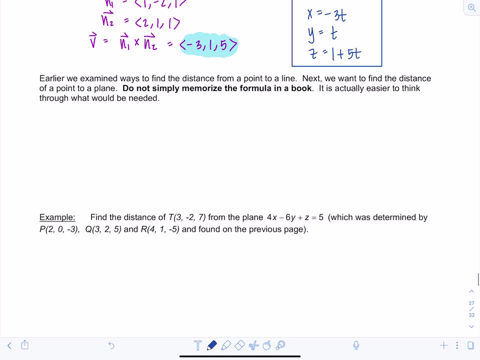 Now, earlier we examined ways to find the distance from a point to a line And I gave you three different methods to do so. Now say I want to actually find the distance from a point to a plane. If you memorize the formula in the book, 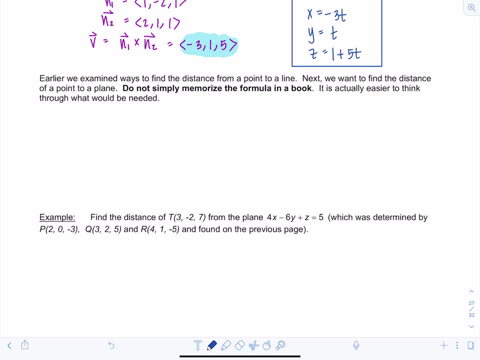 I will give you no credit on a quiz or an exam. Okay, It's actually easier to think through what would be needed and use projections appropriately. So we want to figure out the distance from a point to a plane. So let's think about what we would do. 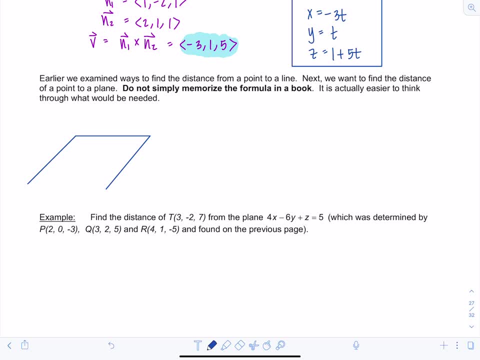 Okay, So here's our plane. I'm not happy with it. Okay, Here's our plane, And I have some point P here. I want to know what the distance is From the point to the plane. Okay, I do have a normal vector because I have the equation of my plane. 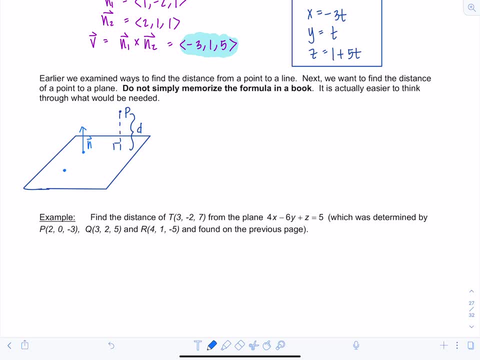 So what would you do? Well, all you would need to do is find any other point on the plane, Any point on the plane. You're going to connect that point on the plane to the point P And what you want to do is project that vector along the normal vector. 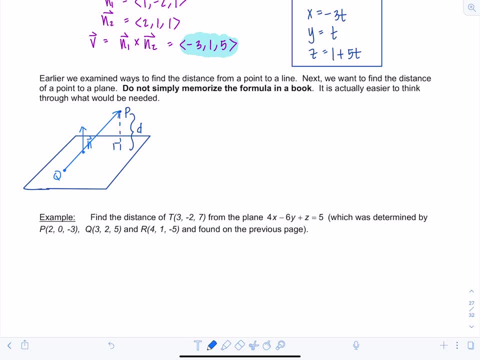 If I project that vector PQ or QP along my normal vector then I will get that distance D, But I want the absolute value of that Right. So the distance D is going to be the absolute value of the scalar projection of the vector PQ along N. 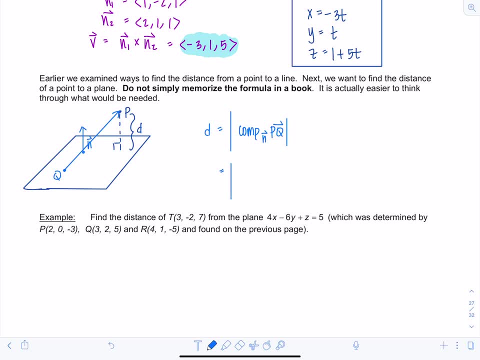 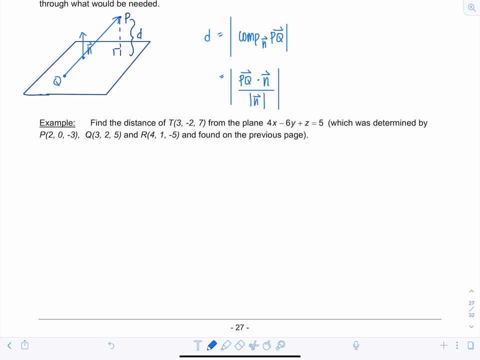 And when you go ahead and compute it, then you would take the dot product of PQ and N And then divide by the magnitude of N. Okay, Good, So let's look at an example, And this would be exactly how I would want you to show it on an exam. 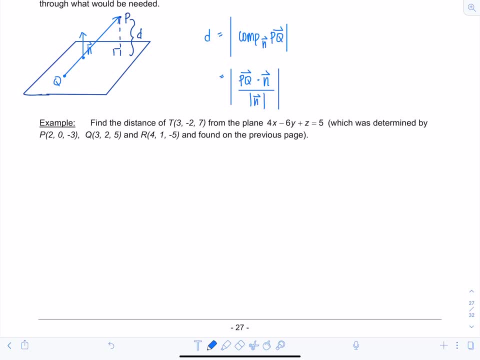 So nice little diagram and notation using the projections, Not some blindly copied formula out of the textbook. So find the distance from the point T to the plane. 4X minus 6Y plus Z equals 5., Which we found previously on the page prior. 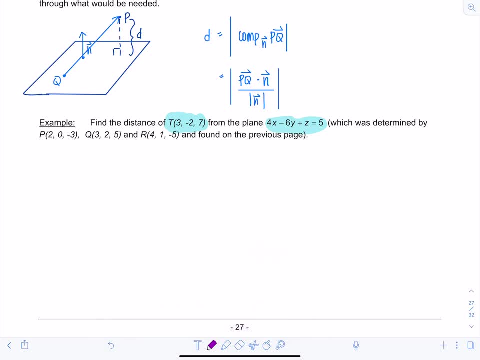 Okay. So first things first, we need to connect T to the plane And in the diagram above I just said we needed one other point that was in the plane. Well, we have an abundance of points. We have three points in the plane.